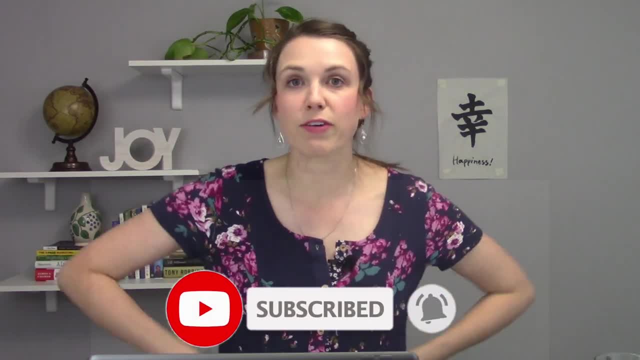 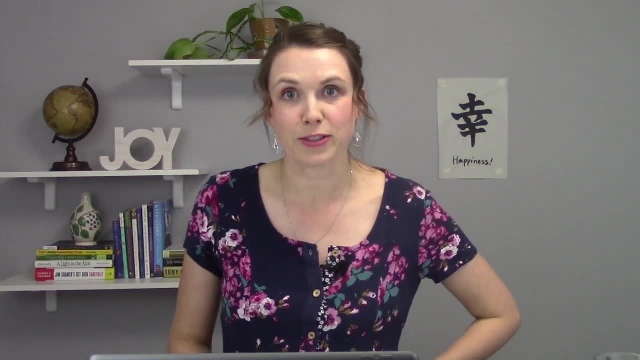 Welcome to our HiSET GED journey. We're just going to have a grand old time here together. Do make sure that you share this video with anyone else that you know that is working on their HiSET or GED. Several folks have asked me if I would provide the slides for the practice test that I'm doing. 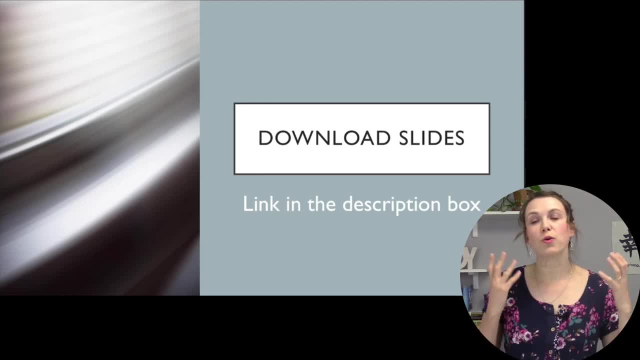 So in the link in the description box down below, you'll be able to access these slides. Now I have them so that you can download for free, or, if you'd like to support my channel. if I am helping you out, help me out too so I can continue. 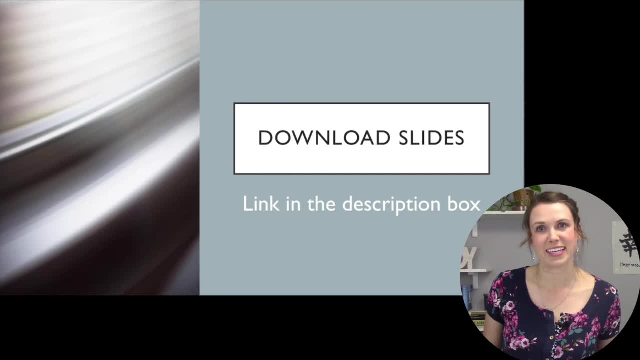 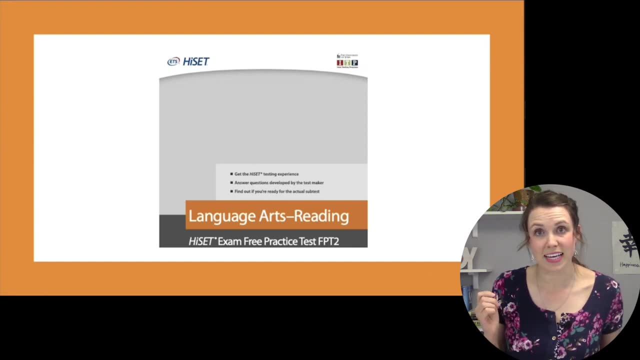 this mission and just pitch in a couple bucks. I definitely appreciate it. Now on with the test. The first several questions that we'll be answering come from the HiSET free practice, test 2.. So I'd like to read the first part, the bolded part, so I really have an idea of what's going on. 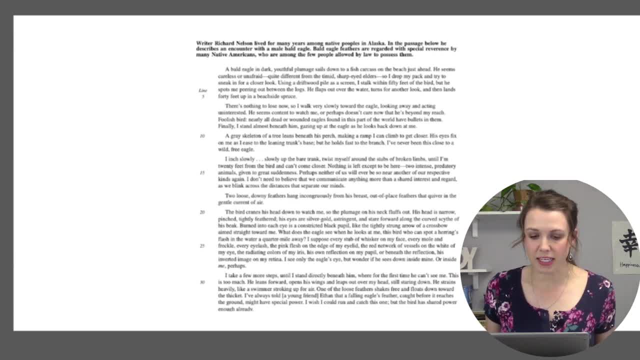 So it says. Writer Richard Nelson lived for many years among native peoples in Alaska. In the passage below he describes an encounter with a male bald eagle. Bald eagle feathers represent are regarded with special reverence by many Native Americans, who are among the few people followed. 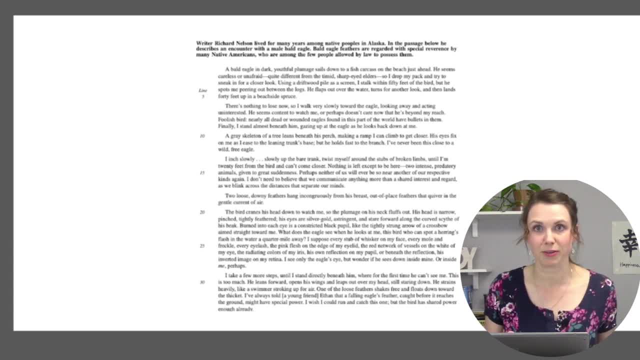 allowed by law to possess them. Oh goodness, I'm having a tough time reading. So then you just want to read a little bit of each of the paragraphs, So I always like to read, maybe just like the first half a line of each paragraph, so I have a general idea of what's going. 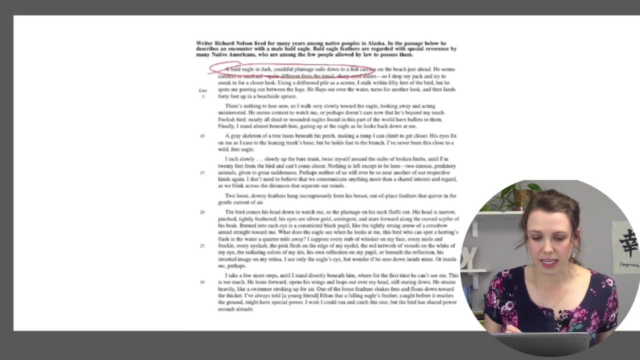 on. So a bald eagle in dark youthful plumage sails down. There's nothing to lose. now A gray skeleton tree leans beneath his perch. I inch slowly. Two loose downy feathers hang. The bird cranes his head down to watch me. I take a few more steps until I stand directly beneath him. Okay, so we have a. 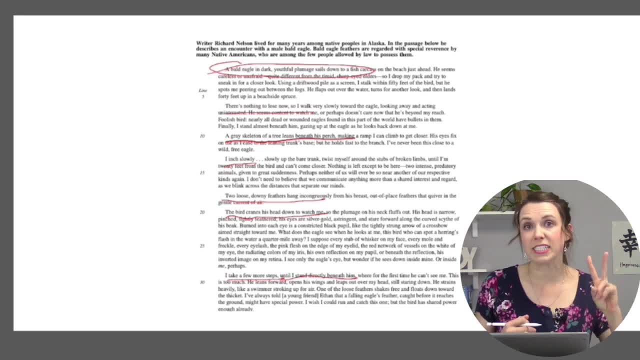 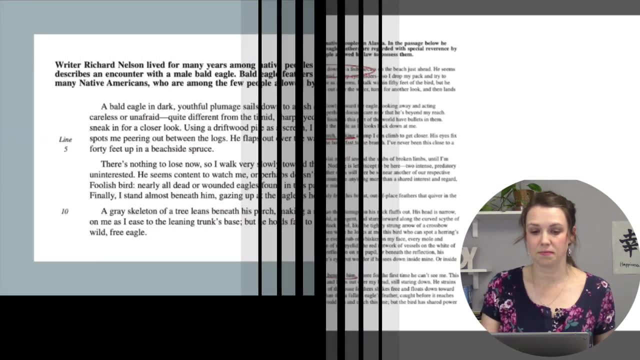 general idea of what's going on. So we start with survey, then I would normally take a look at the questions, but I'm not going to do that here. I'm actually just going to go right into reading. So I'm going to read the actual article, but I already read the bolded part, so I'm just going to go. 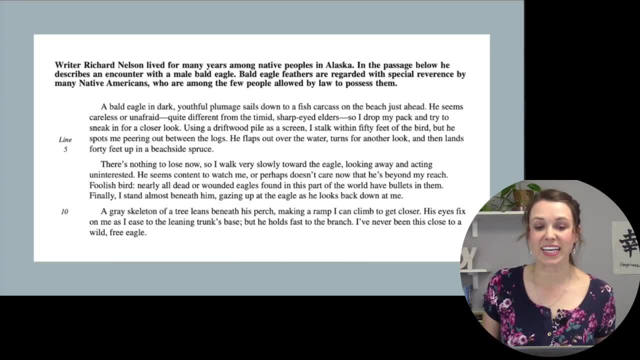 straight to the article. A bald eagle in dark youthful plumage sails down to a fish carcass on the beach just ahead. He seems careless or unafraid, quite different from the timid, sharp-eyed elders. So I drop my pack and try to sneak in for a closer look Using a driftwood. 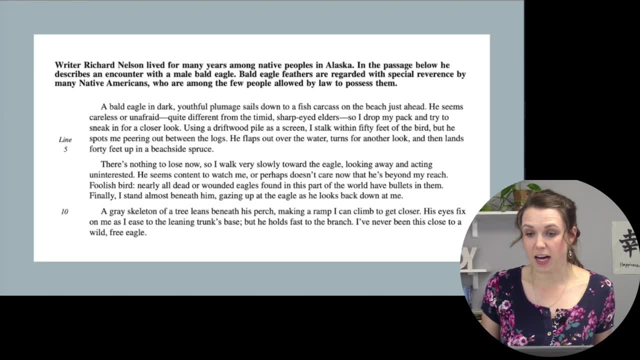 pile as a screen. I stalk within 50 feet of the bird, but he spots me peering out between the logs. He flaps out over the water, turns for another look and then lands 40 feet up in a beachside spruce. There's nothing to lose now. I walk very slowly. 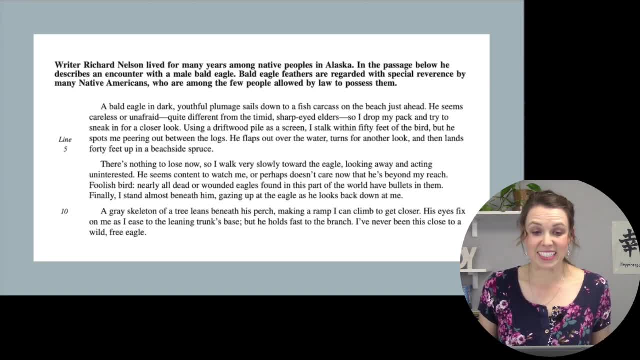 toward the fish carcass, Looking away and acting uninterested. he seems content to watch me, or perhaps doesn't care now that he's beyond my reach. Foolish bird. Nearly all dead or wounded eagles found in this part of the world have bullets in them. Finally, I stand almost beneath him, gazing up at the eagle as he 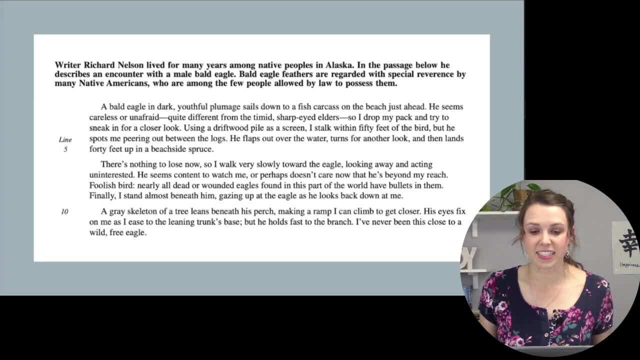 looks back down at me. A gray skeleton of a tree leans beneath his perch, Making a ramp I can climb to get closer. His eyes fix on me as I ease to the leaning trunk's base, But he holds fast to the branch. I've never been this close to a wild free eagle. 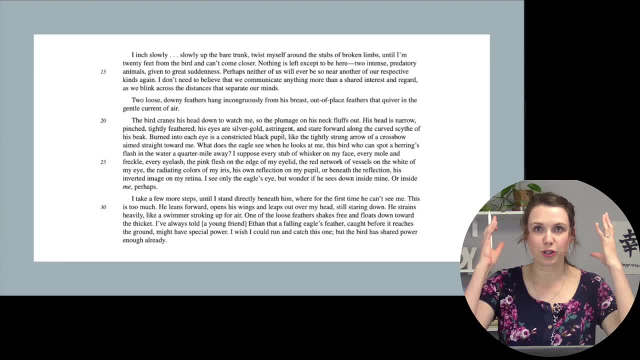 So, as I'm reading this, try to picture it in your head. If you can create an image in your head of what is going on, kind of like a movie, it will really help you better comprehend what is going on in your head. So I'm going to try to picture it in my head. I'm going to try to. 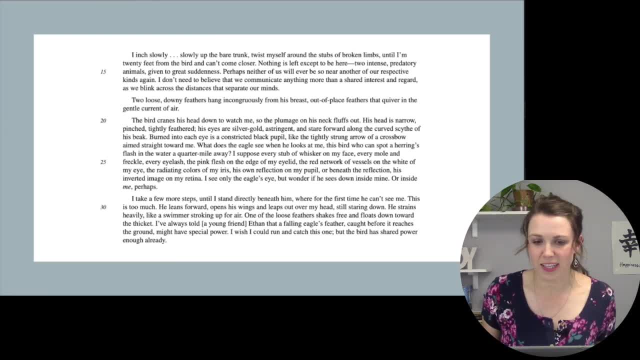 create an image of what it is that's going on in this story. I inch slowly, slowly up the bear trunk, twist myself around the stubs of broken limbs until I'm 20 feet from the bird and can't come closer. Nothing is left except to be here: Two intense predatory animals given to the great. 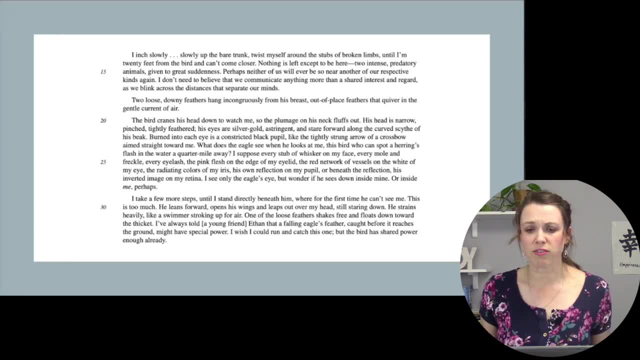 suddenness. Perhaps neither of us will ever be so near another of our respective species. I don't need to believe that we communicate anything more than a shared interest and regard. as we blink across the distances that separate our minds, Two loose downy feathers hang. 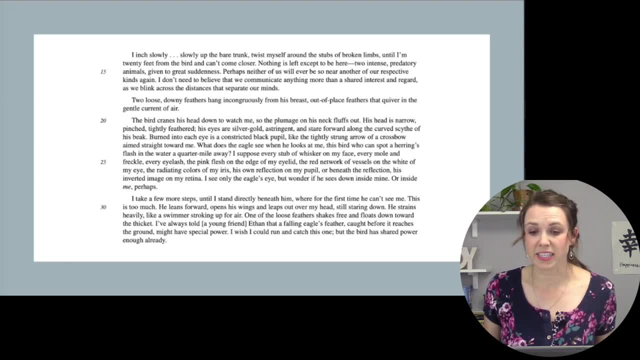 incongruously from his breast, Out of place, feathers that quiver in the gentle current of air. The bird cranes his head down to watch me, so the plumage on his neck fluffs out. His head is narrow, pinched, tightly feathered. His eyes are silver-gold, astringent and stare. 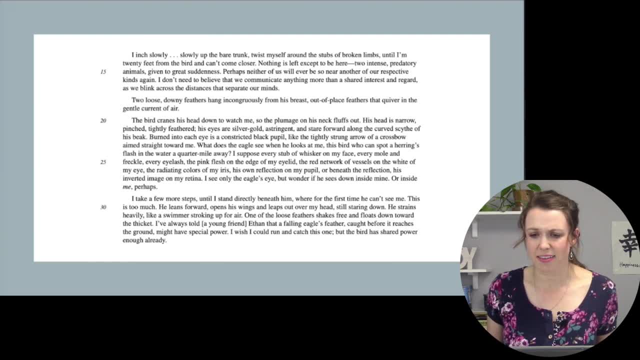 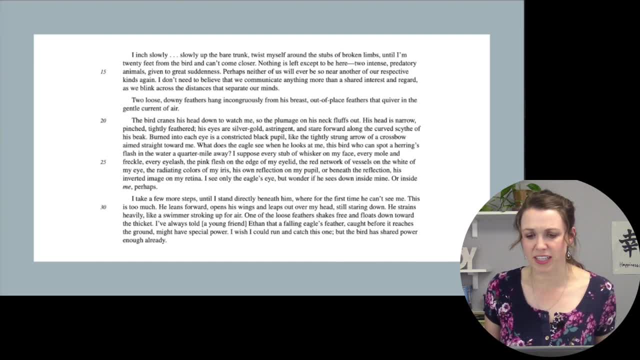 I suppose every stub of whisker on my face, every mole and freckle, every eyelash and the pink flesh on the edge of my eyelid, the red network of vessels on the white of my eye, the radiating colors of my iris, his own reflection on my pupil or, beneath the reflection, his inverted image on 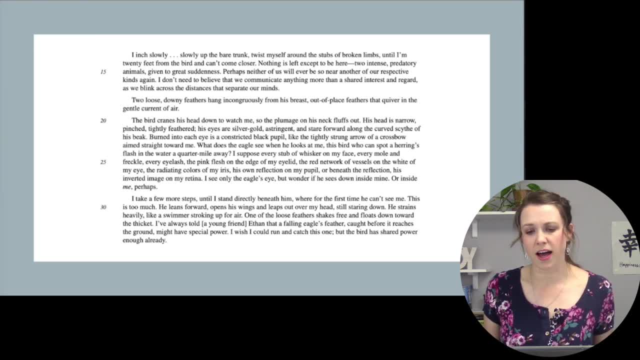 my retina I see only the eagle's eye, but I wonder if he sees down inside mine or inside me. perhaps I take a few more steps until I stand directly beneath him, where, for the first time, he can't see me. This is too much. He leans forward, opens his wings and leaps out over my head, still staring down. 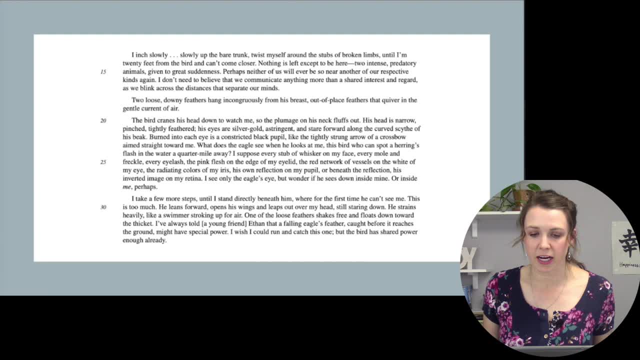 He strains heavily like a swimmer stroking up for air. One of the loose feathers shakes free and floats down toward the thicket. I've always told a young friend, Ethan, that a falling eagle's feather, caught before it reaches the ground might have a special power. 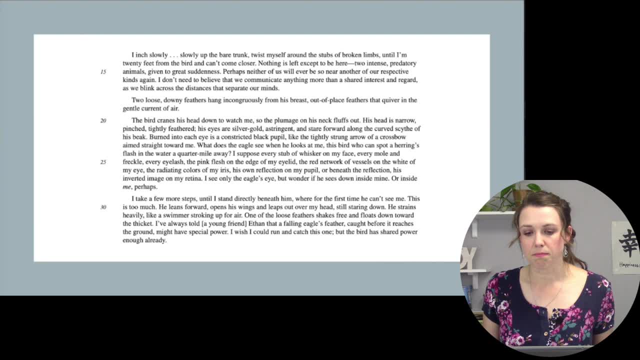 I wish I could run and catch this one, but the bird has shared power enough already, Alright. so hopefully you envisioned that story and really comprehended it well, since it was like a movie in your brain, hopefully. Okay, our first question here. 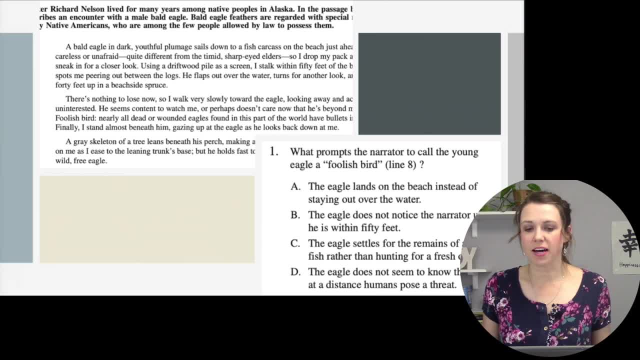 What prompts the narrator to call the young eagle a foolish bird in line 8?? So usually you can see where it says line 8, but in this case we can't but right here. So it says foolish bird. nearly all dead or wounded eagles found in this part of the world have bullets in them, right? 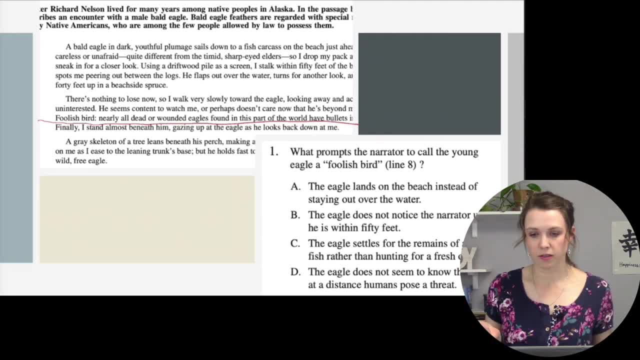 So why is he calling the young eagle a foolish bird? Because so A the eagle lands on the beach instead of staying out over the water. That's not really why he's a foolish bird. right, The eagle does not notice the narrator until he is within 50 feet. 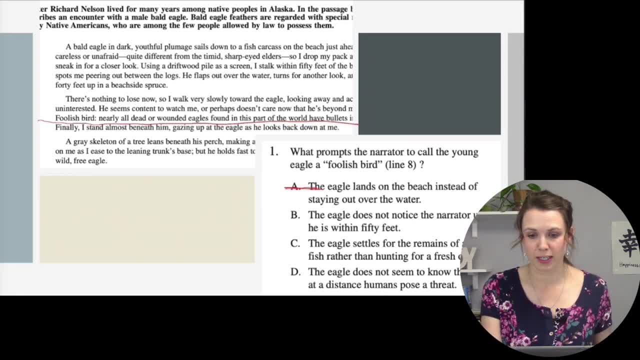 Now it's kind of indicating that the eagle is very aware of the narrator. right, The eagle settles for the remains of a dead fish rather than a dead bird. The eagle settles for the remains of a dead fish rather than a dead bird. 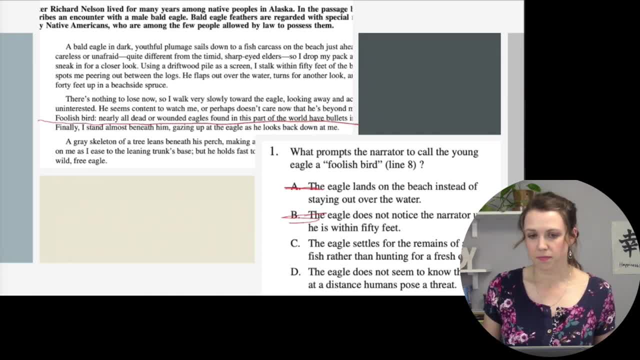 The eagle settles for the remains of a dead fish rather than a dead bird. The eagle is now in hunting for a fresh one. I mean, it does talk about how there's the dead fish carcass right. It talks about that in the very first line. 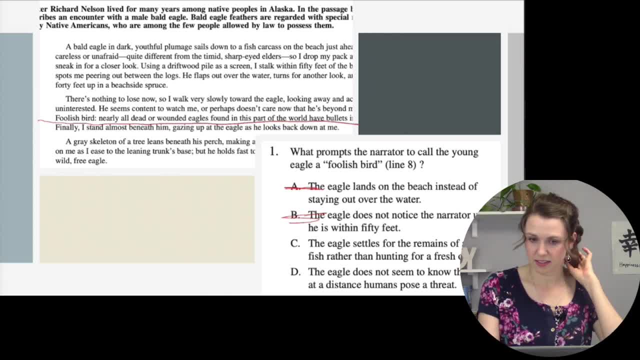 But that's not why he's a foolish bird, right? Because I mean, we're really talking about humans, right, And the bullets that are in an eagle, if they're ever this close. So the answer here is D. 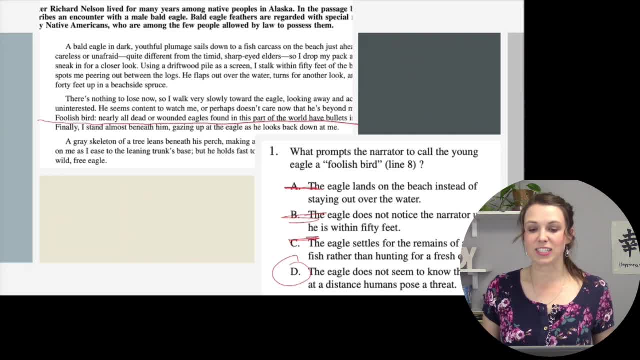 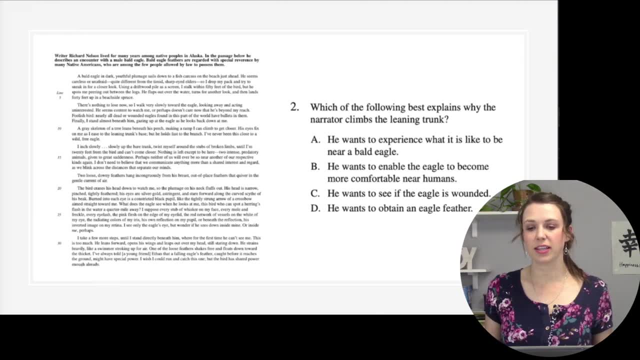 The eagle does not seem to know that even at a distance, humans pose a threat. Number 2.. the following best explains why the narrator climbs the leaning trunk. So right, he's climbing the trunk, He's just trying to get kind of close to the eagle, right. So he wants to experience what 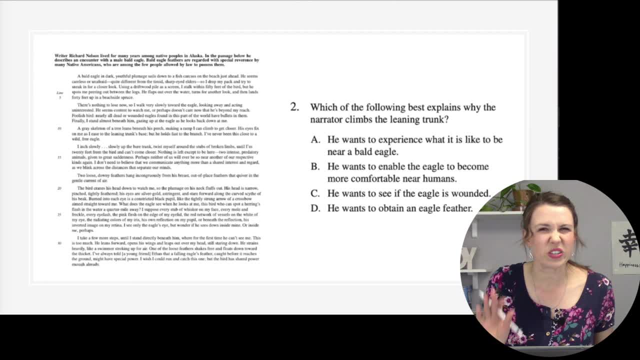 it is like to be near a bald eagle. Sure, right, Let's look at the other ones too. He wants to enable the eagle to become more comfortable near humans. Is it really about how he wants the eagle to be comfortable with humans or is it more sort of selfish? He wants to be near a human. 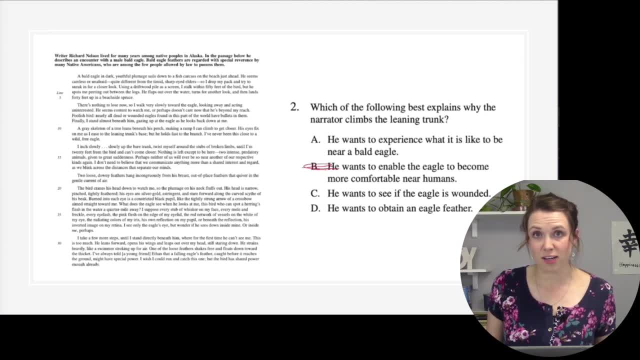 right, So it's not B. He wants to see if the eagle is wounded. No, it doesn't really talk about the eagle being wounded at all, right, If it did, then maybe it would talk about, like the eagles having issues flying, that sort of thing. So it's. 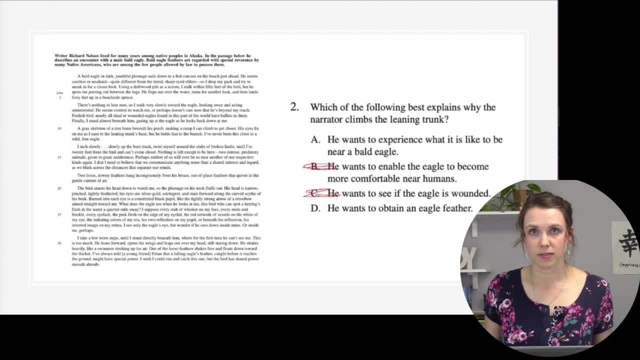 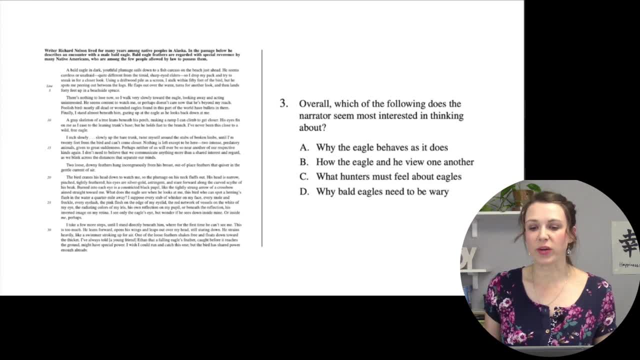 can right Number three Overall. which of the following does the narrator seem most interested in thinking about Why the eagle behaves as it does? It talks a little bit about the eagle's behavior, but it's not really what the narrator is interested in. right The narrator? 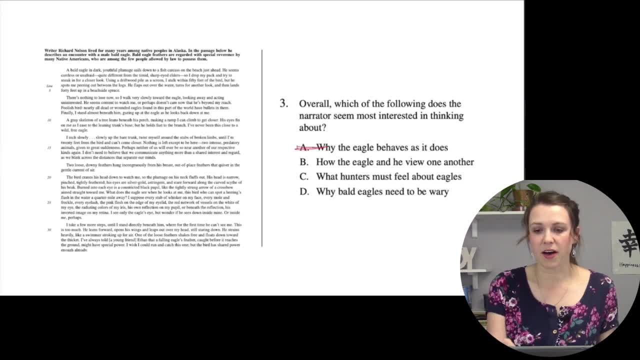 probably knows eagles pretty well, but how the eagle and he view one another. it does talk about that, right. It talks about how the eagle is seeing into the narrator, like he can see every whisker, every freckle, the white of his eyes, the pink of the skin. 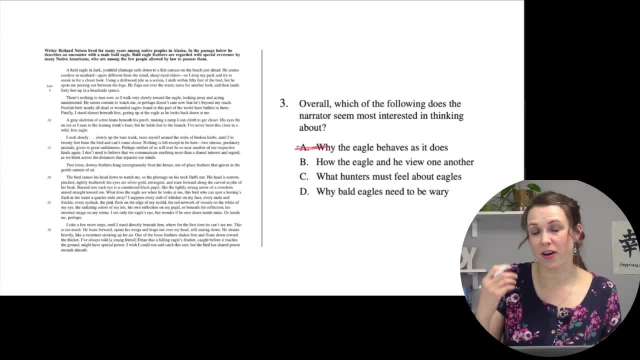 with his eyelashes, right. It's really going into depth on how the eagle is viewing him, but then also how he views the eagle right. So definitely B, but let's look at the the other answers too, How hunters must feel about eagles. He's not really thinking about. 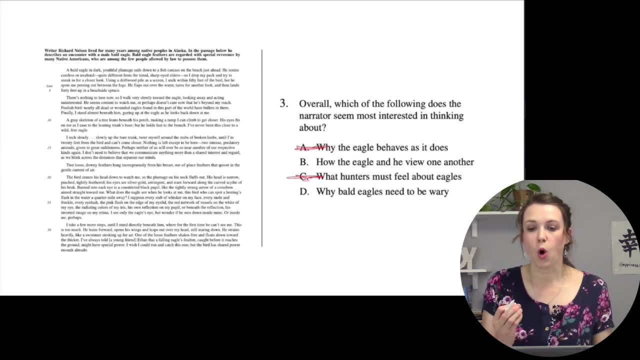 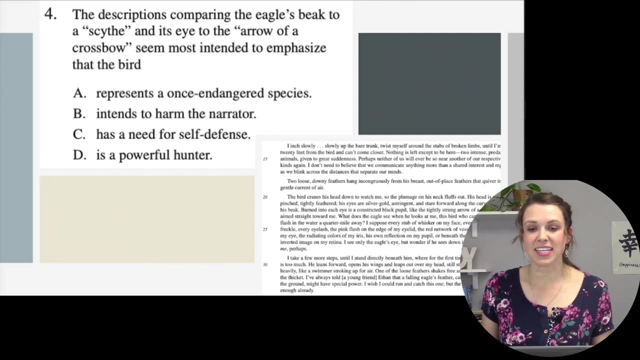 hunters and eagles. right, He's just trying to embrace this eagle. Why bald eagles need to be wary? He knows why they need to be wary, He just really wants to. he's thinking about how they're viewing each other. The descriptions comparing an eagle's beak to a scythe and its eye to the 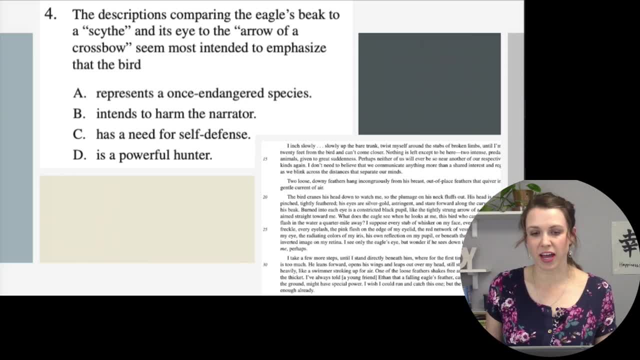 arrow of a crossbow seem most intended to emphasize that. the bird. okay, so a scythe. if you don't know what a scythe is, that's like the grim reaper. He has like a that special like knife, sword, sword type thing. It kind of like a machete sort of, but angled. 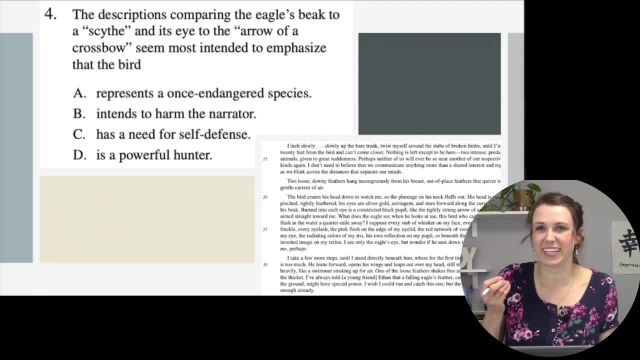 like that kind of like the bird's beak right Sort of indicating depth, And then the arrow of a crossbow also kind of angled. you know, crossbow is what somebody uses when they're hunting, right? So both of those descriptions comparing the eagle's beak and the eye, 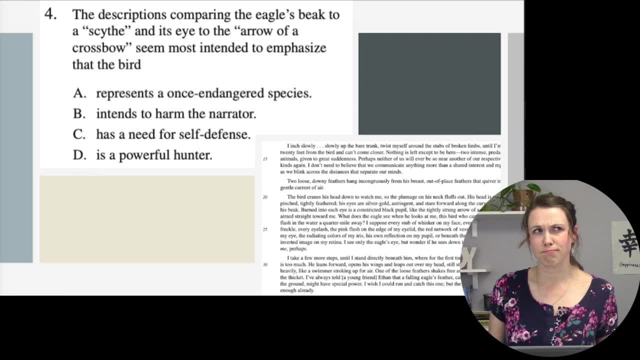 so they represent a once endangered species, Not so much. Those aren't really talking about endangered species, right? Intends to harm the narrator Again. it's just explaining. this is how the bird looks. Has a need for self-defense. Are eagles aiming for self-defense? No, No. 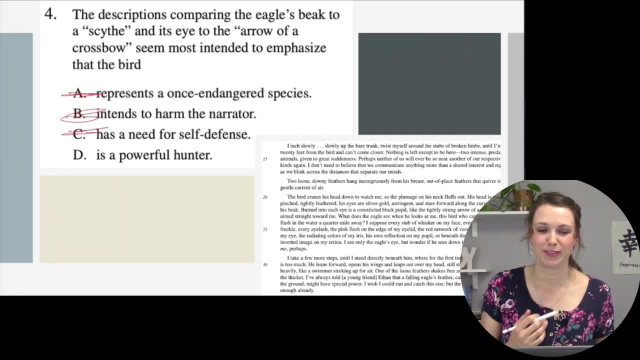 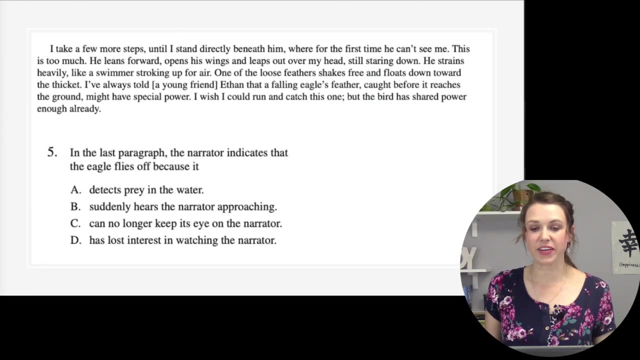 because they're top of the food line, right Or close to the top of the food chain. A powerful hunter right, A scythe and a crossbow are like that, right, That's what hunters could use. So there we go, The easy answer. In the last paragraph, the narrator indicates that the eagle 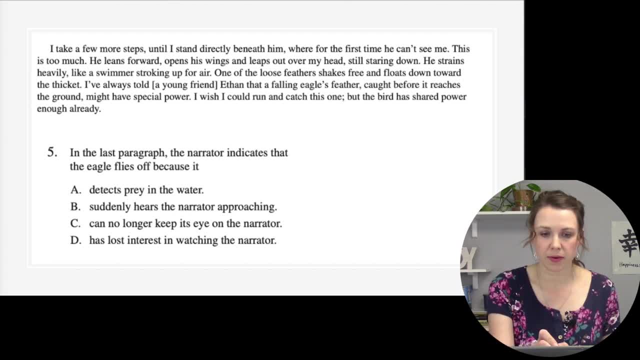 flies off because it so. here we can actually see it's right in these first sentences, right? So let's reread that part. So is he flying away because he detects prey in the water? No, Because he hears the narrator approaching. He knows that the narrator is approaching. 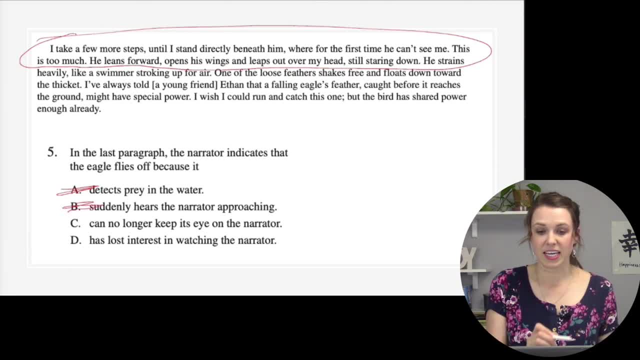 right. He's been keeping a close eye on the narrator. He can no longer keep his eye on the narrator. that's, that's it right. because it says right here for the first time: he cannot see me. so there we go. and is he lost interest? not really. he just can't see the narrator. he doesn't know what's. 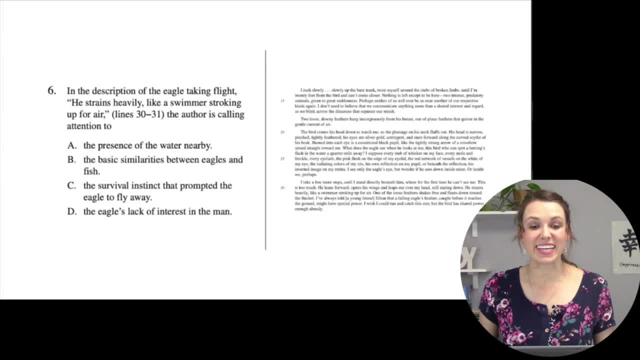 going on. so he's like i'm out of here. right number six in the description of the eagle taking flight. he strains heavily like a swimmer stroking up for air the author is calling attention to. so before we go any further again, if you haven't already downloaded the slides, definitely make. 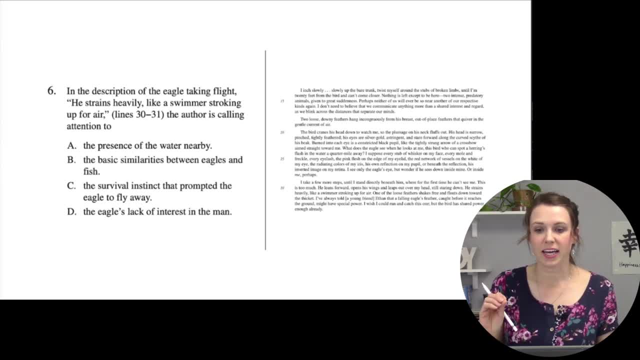 sure that you do. it's just right in the description box for the link, and this will make it a lot easier to see. i wasn't able to make this one much bigger, so we don't really need it as much for the to answer this question, but having those slides will really help you. okay, so again, he strains heavily. 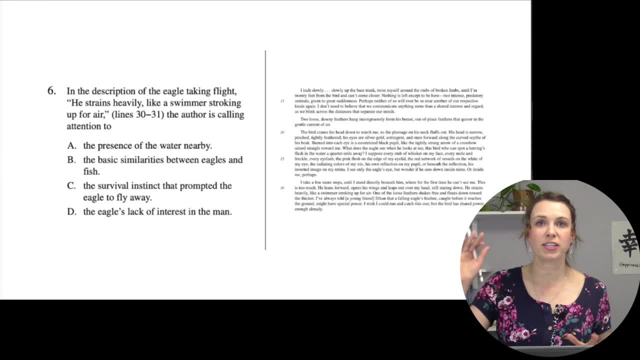 like a swimmer stroking up for air. so just imagine a swimmer, right, a swimmer is swimming and then a swimmer leans his head over, her head over and breathes right, gets gets more air, right. we have to do that in order to be able to breathe while we're swimming, right, and survive okay. so, as it's talking about, 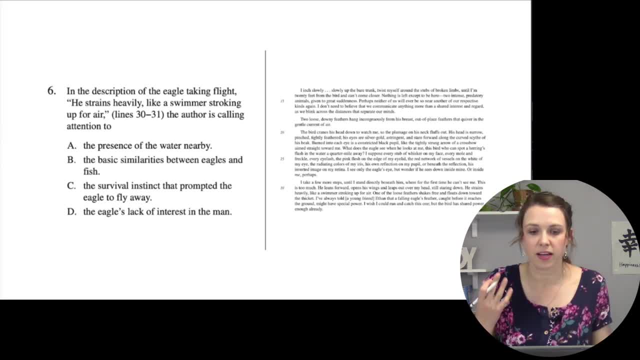 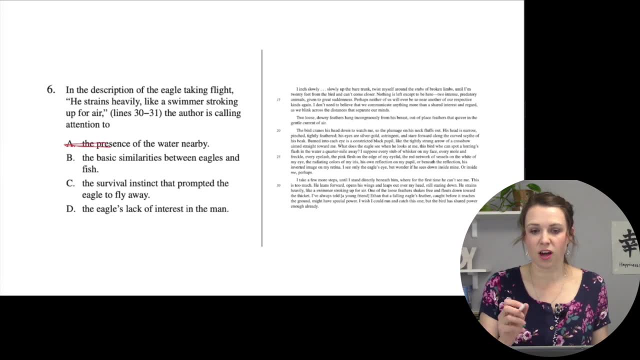 that the eagle is flying, and then he does that, right. so the presence of water nearby? um, that one's trying to trick you, right, because it's talking about a swimmer, oh, that must mean water, right, but that's not actually the case. the basic similarities between eagles and fish. we're not talking about fish. 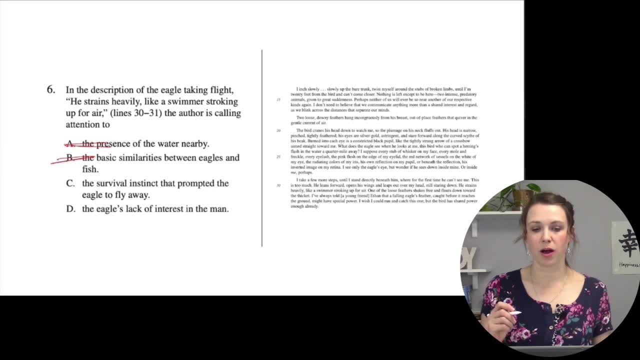 the survival instinct that is prompt, that prompted the eagle to fly away. right, isn't a swimmer stroking up for air? imagine somebody swimming. it's like instinct. you have to get your head out of the water so that you can breathe. right, just like it's a survival instinct. 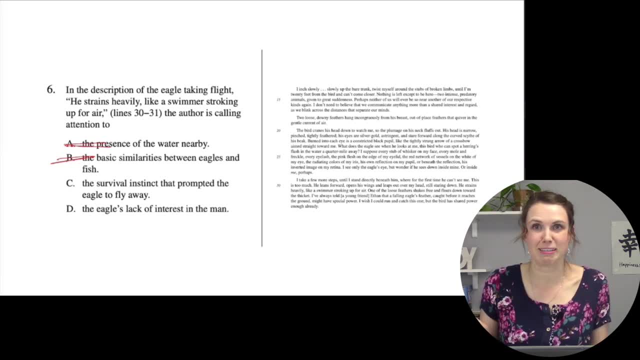 if you don't get up to breathe, then you're not going to survive, right? so, uh, c's the answer here, and d doesn't really have anything to do with. there's no comparison of the lack of interest, and a swimmer is trying to breathe, right? so c is the answer. this question here is: it's an analysis. 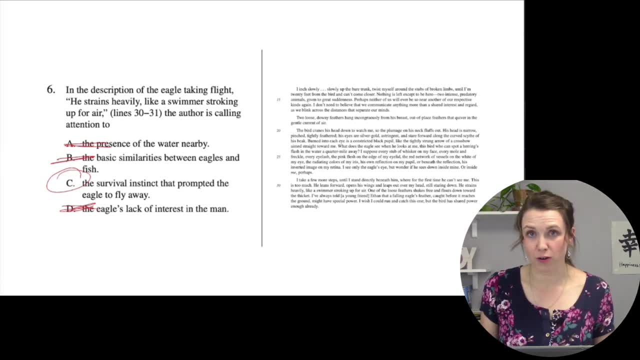 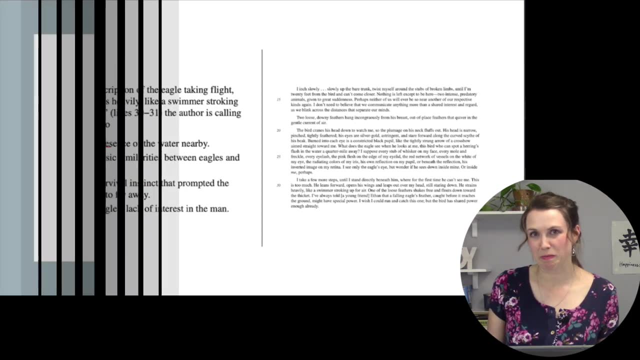 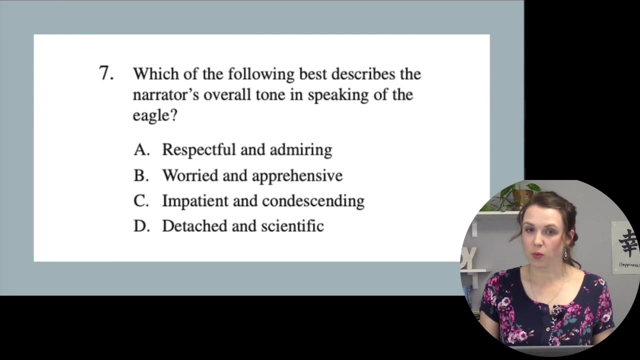 question and it's actually marked as difficult. so hopefully, by me answering this question and going through it with you, hopefully it helps you understand it just a little bit better. which of the following best describes the narrator's overall tone in speaking of the eagle: respectful and admiring? yes, right, he was definitely admiring the eagle and being respectful, right. 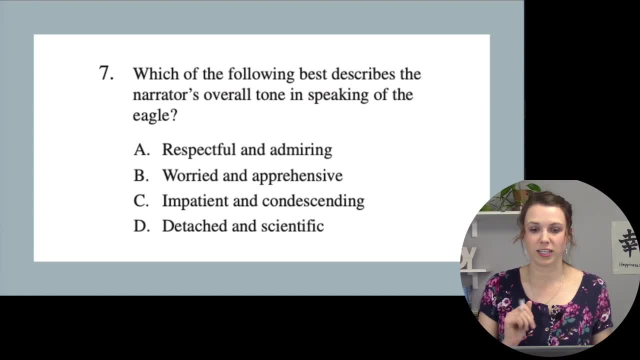 he was just there watching the eagle. right, was he worried and apprehensive? not really, he was just really curious. right was he impatient and condescending. he was sitting there for a little while. i would call that patience, detached and scientific. was he detached he? no, he had this like special, unique bond with the eagle right. 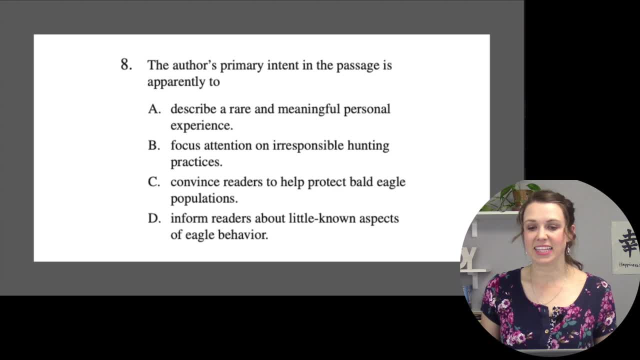 so our answer is a. the author's primary intent in this passage is apparently to inspire people to think creatively about regards to lies. doesn't really mean much at all, but i'm not sure. but i would say it actually was a lot of things that he did. 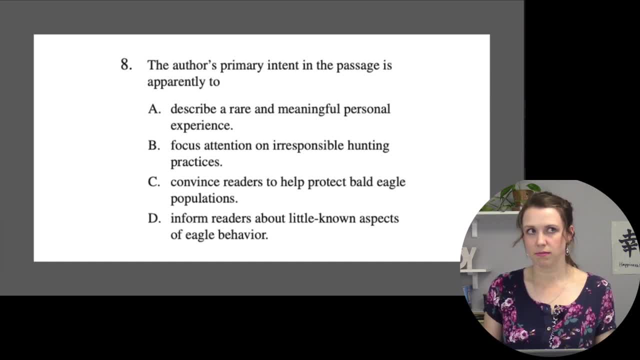 that saw a deep effect on people like himself and knowledge was really big in the way that he was describing in this passage. he was saying: you know it's, you know, would you remember, good friends, don't bring spanish for your visit, like in contraband. you know, say you had this. 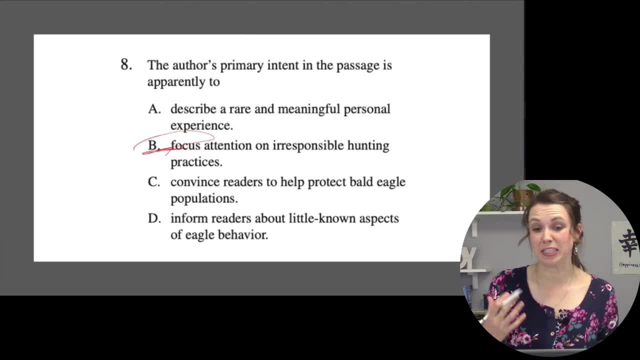 participate in black market areas where white people shouldn't have come over for public transformer, trying to convince anyone right Inform readers about little known aspects of ego behavior. No, this was really just about this personal experience that the author had. I've said this in past videos. 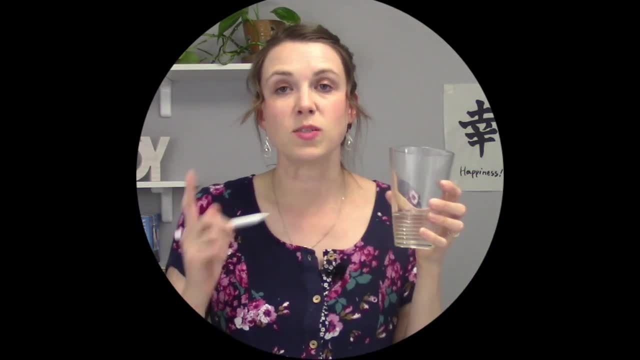 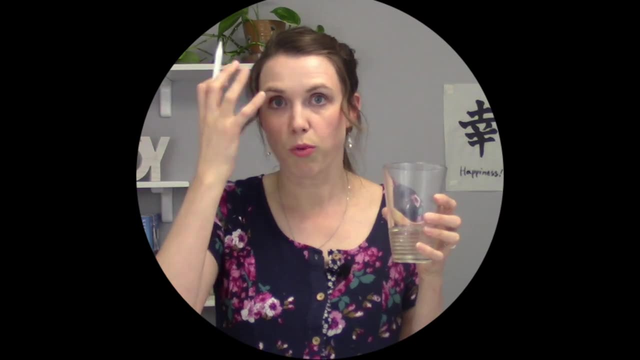 but you definitely wanna make sure that you're drinking lots of water, especially the day before you take your test, so that your brain is fully hydrated and you can reach the outer portions of your brain. that is going to help you do better on the test. 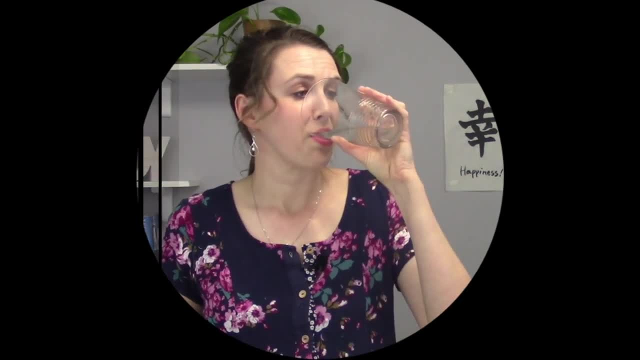 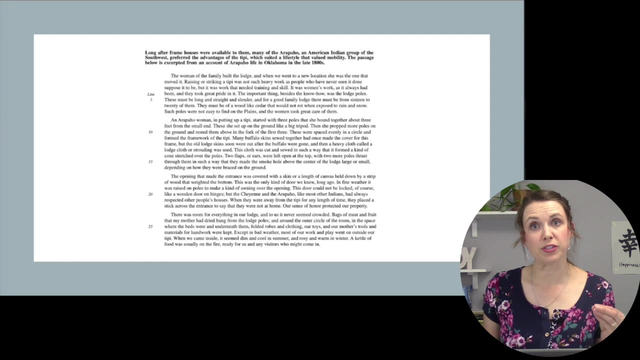 So definitely make sure to drink up. So here's another little practice passage for us. So we'll start with surveying and then we'll go jump into those questions. Long after frame houses were available to them, many of the Arapaho and American Indian group. 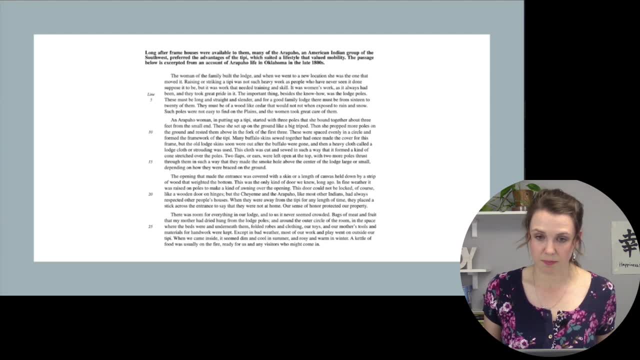 of the Southwest prefer the advantage of the teepee, which suited a lifestyle that valued mobility. The passage below is excerpted. excerpted from an account of Arapaho life in Oklahoma in the late 1800s. So again, I'm going to read just the first, like half a line. 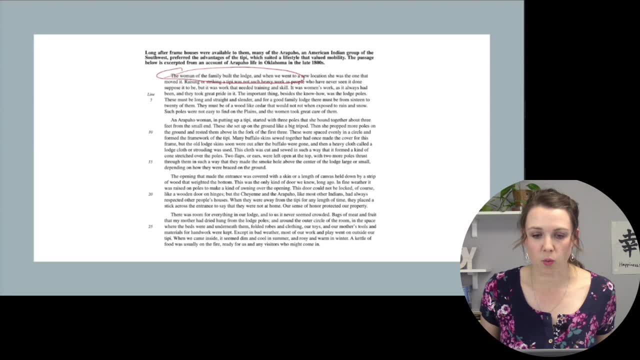 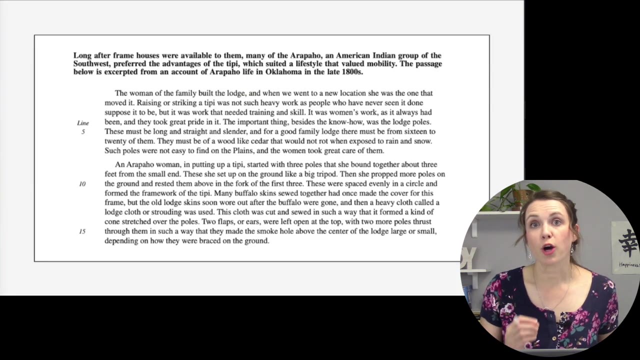 Women of the family built the lodge- An Arapaho woman in putting up a teepee. The opening that made the entrance was covered with the skin. There was room for everything in our lodge. Okay, so at this point I would normally go right in. 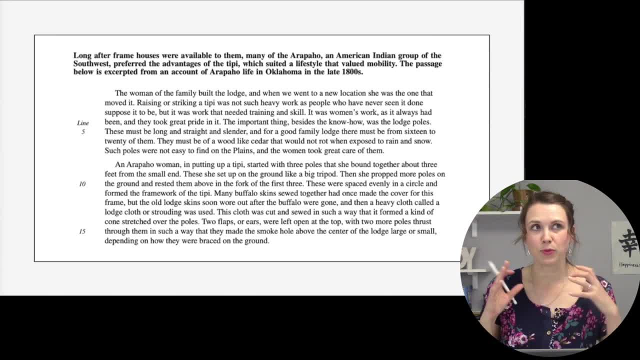 and just take a quick survey of the questions, And you want this whole process of surveying- just sort of seeing what's going on and answering the questions- to take maybe 30, 45 seconds, because it is a time test, but then you have a little bit more purpose. 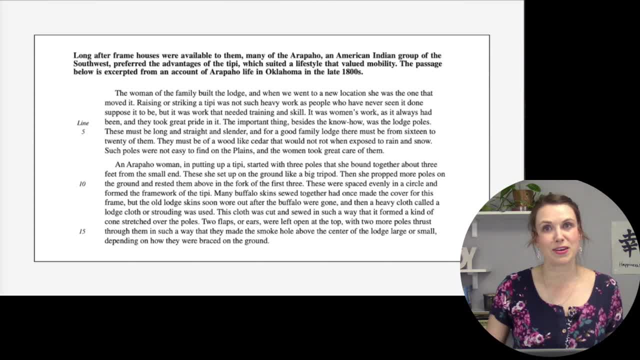 and an idea when you're reading, But let's get to the article and actually read it. So you said this one match for you. I think there's a big answer for this question. The women of the family built the Lodge, and when we went to a new localatio, 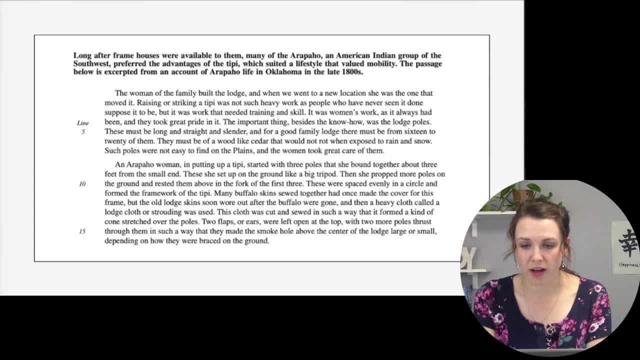 she was the one that moved it. Rising or striking a teepee was not such heavy work as people who have never seen it done supposed it would be, But it was work that needed training and skill. It was women's work. The important thing besides the know-how was the lodge poles. 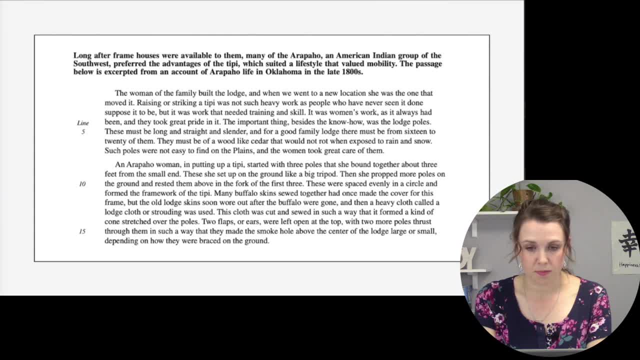 These must be long and straight and slender, And for a good family lodge there must be from 16 to 20 of them. They must be a wood-like cedar that would not rot when exposed to rain and snow. Such poles were not easy to find on the plains. 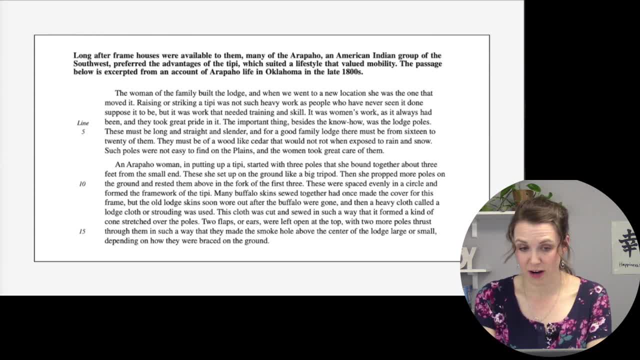 And the women took great care of them. An Arapahoe woman, in putting up a teepee, started with three poles that she bound together about three feet from the small end. Then she set up on the ground like a big tripod. 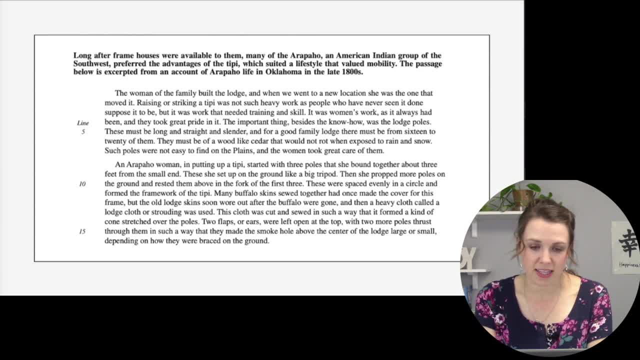 Then she propped more poles on the ground and rested them above in the fork of the first three. These were spaced evenly in a circle And formed the framework of the teepee. Many buffalo skins sewed together had once made the cover for this frame. 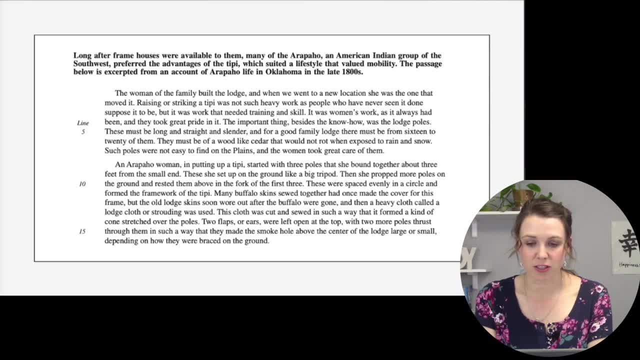 But the old lodge skins soon wore out after the buffalo were gone, And then a heavy cloth called the lodge cloth or strouting was used. This cloth was cut and sewed in such a way that it formed a kind of cone stretched over the poles. 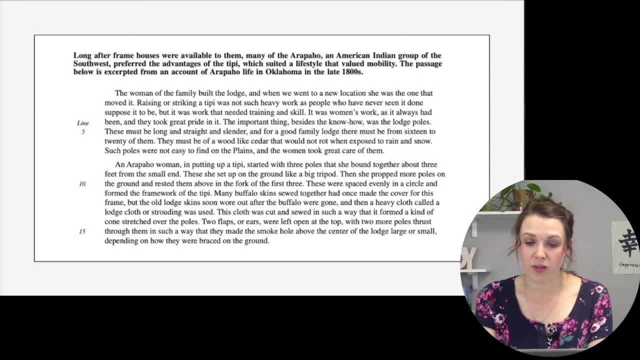 Two flaps or ears were left on top of the poles. Two flaps or ears were left on top of the poles. Two flaps or ears were left on top of the poles. Two flaps or ears were left open at the top, with two more poles thrust through them in such a way that they made the smoke hole above the center of the lodge large or small, depending upon how they were braced on the ground. 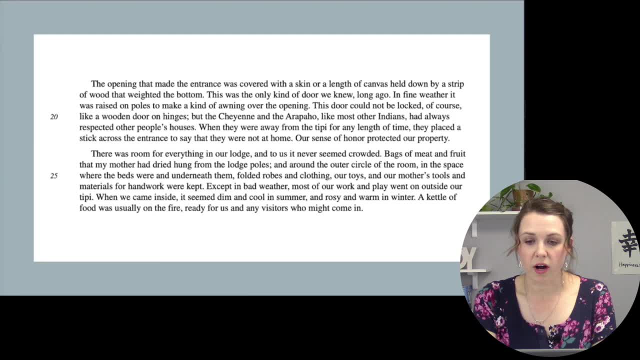 The opening that made the entrance was covered with a skin or a length of canvas, held down by a strip of wood that weighed the bottom. This was the only kind of door we knew long ago. In fine weather it was raised on poles to make a kind of awning over the opening. 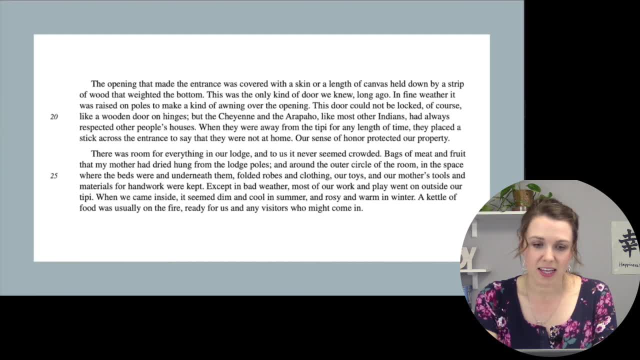 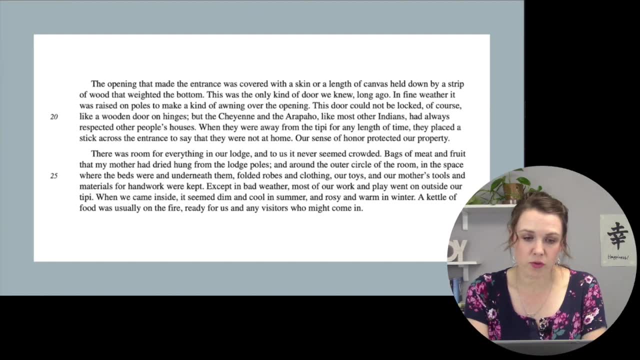 This door could not be locked, of course, like a wooden door on hinges, But the Cheyenne and Arapaho, like most other Indians, had always respected other people's houses. When they were away from the teepee for any length of time, they placed a stick across the entrance to say they were not at home. 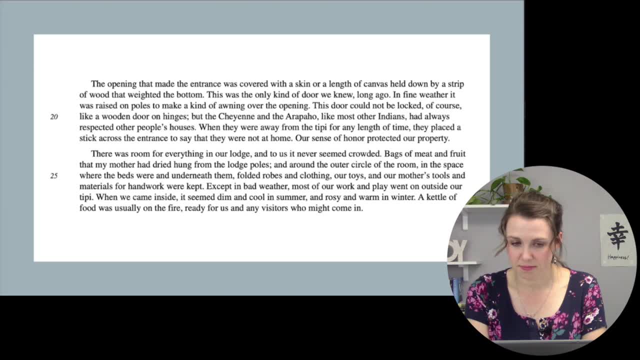 Our sense of honor protected us. Our sense of honor protected our property. There was room for everything in our lodge, And to us it never seemed crowded. Bags of meat and fruit that my mother had dried hung from the lodge poles And around the outer circle of the room, in the space where the beds were and underneath them, folded robes and clothing. our toys and our mother's tools and materials for handiwork were kept. 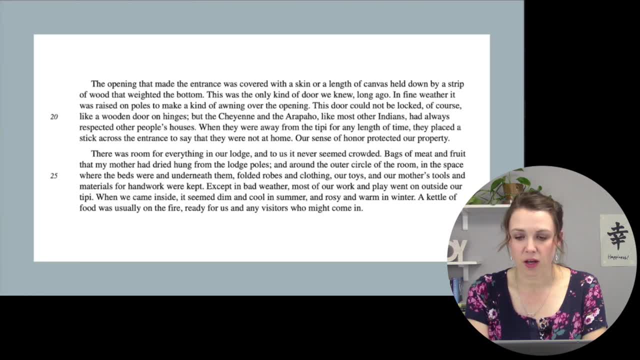 Except in bad weather, Most of our work and play went on outside our teepee. When we came inside, it seemed dim and cool in summer and rosy and warm in winter. A kettle of food was usually on the fire ready for us and any visitors who might come in. 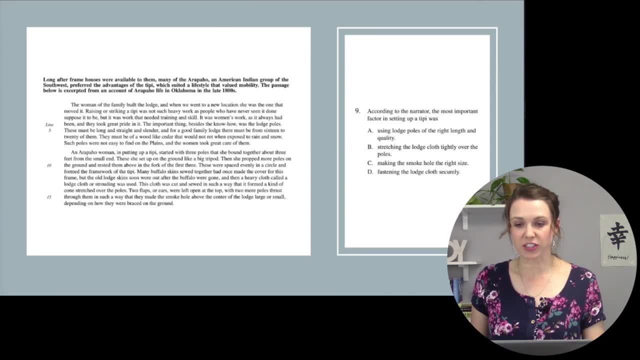 According to the narrator, the most important factor in setting up a teepee was- and you can see here it's right here in this first paragraph. So it says The important thing besides the know-how was the lodge poles, right? So it really goes into detail on the lodge poles, the length, what it's made of, where to find it or, I guess, where not to find it, that sort of thing right. 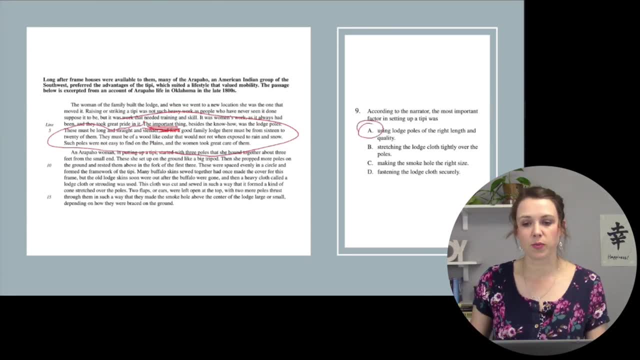 So we know here the answer is A, but let's look at the other ones as well. So: A- using lodge poles the right length and quality. B- stretching the large cloth tightly over the poles. C- making the smoke hole the right size. 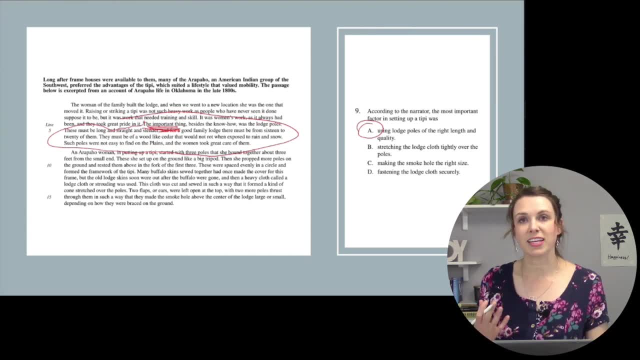 Or D, fastening the lodge cloth securely. So definitely A. This was a bit of an easier question, but a lot of times the most important thing is mentioned first right, And in this case it definitely was 10.. 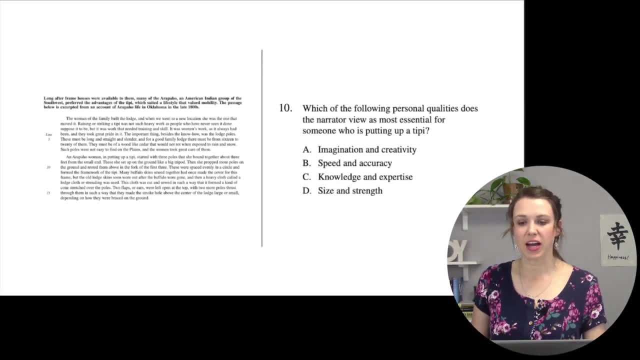 Which of the following personal qualities does the narrator view as the most essential for someone who is putting up a teepee? Imagination and creativity. Do you need imagination when setting up a teepee? Do you need to be creative? No, you need to do what you're supposed to do, right. 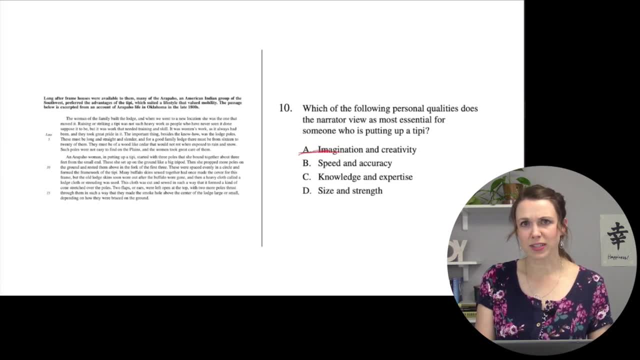 Speed and accuracy. It doesn't really talk about speed, right. It doesn't say you need to put it up quickly. It just really talks about- there we go C knowledge and expertise. You've got to know how to put it up and be an expert at putting it up right. 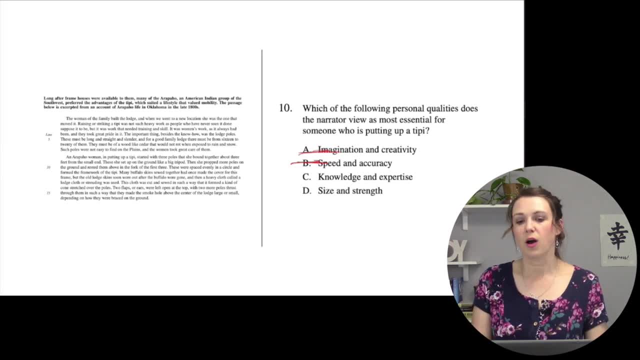 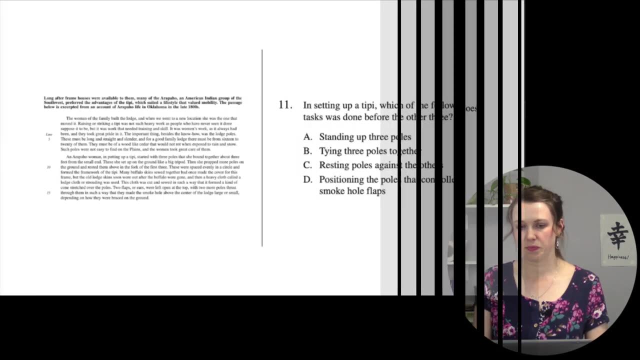 This is where we're going to live. We want to make sure that those ladies know what they're doing. D size and strength- No, it doesn't really talk about that. Mostly We see that knowledge and expertise 11.. 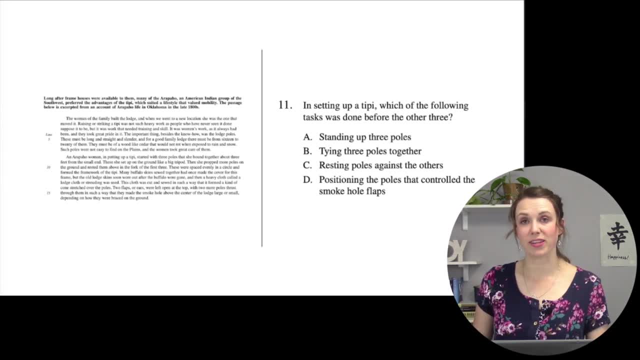 In setting up a teepee, which of the following tasks was done before the other three? Okay, so standing up the three poles, tying three poles together, resting poles against the others or positioning the poles that controlled the smoke hole flaps. 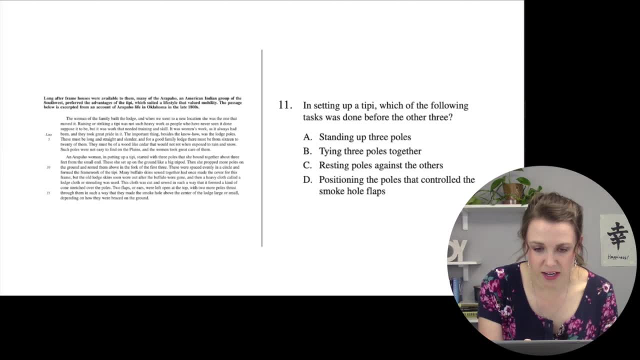 So in this one here you have to go into it And it's, It's right here. So it says an Arapaho woman, in putting up a teepee, started with three poles that she bound together about three feet from the small end right. 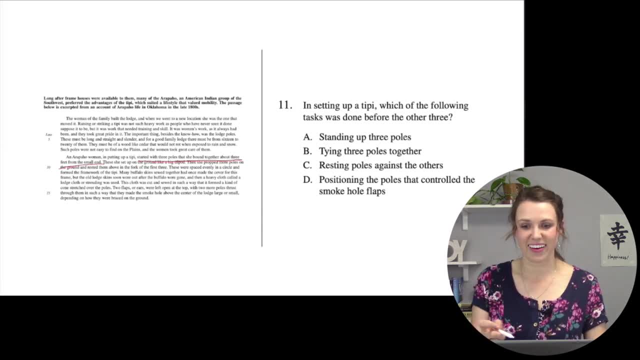 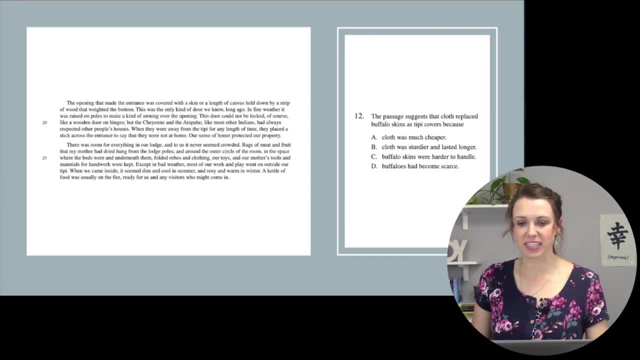 Number 12. Number 12.. Number 12.. The passage suggests that cloth replaced buffalo skins as teepee covers, because cloth was cheaper. You know they weren't buying the buffalo skins, right? They were hunting the buffalo skins, So it wasn't really a matter of cost. 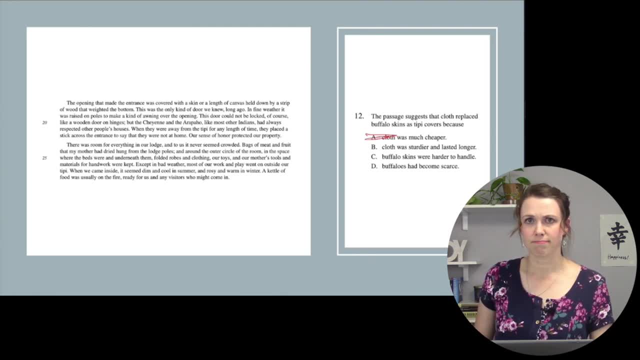 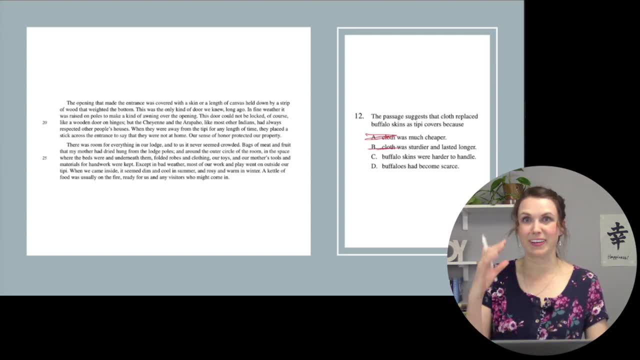 Right, Right, Right. It sounded like the cloth. you could wrap around it a little bit better. But D says buffalo had become scarce. Yeah, that's what it talked about, right, It talked about how the buffalo were becoming more scarce in the Great Plains, where they 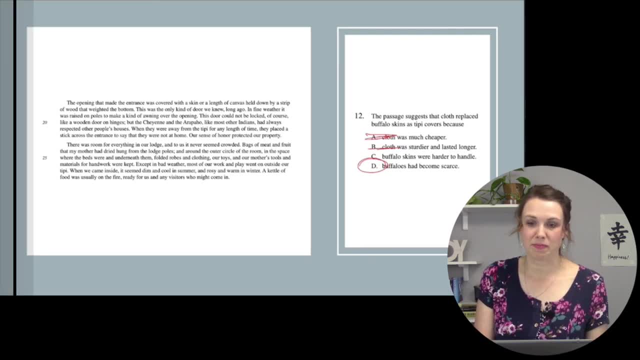 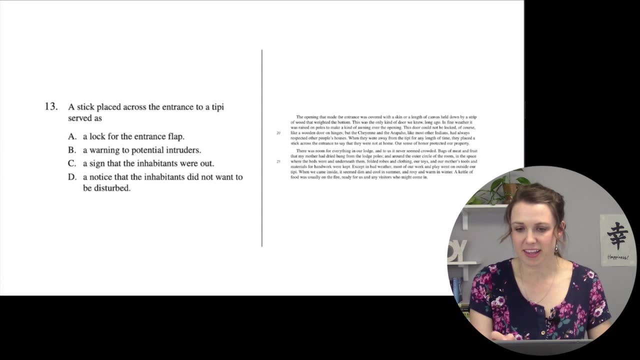 had the teepees right, Number 13.. A stick placed across the entrance of a teepee served as, do you remember? we read that So right here. Here is where it says: when they were away from the teepee for any length of time. 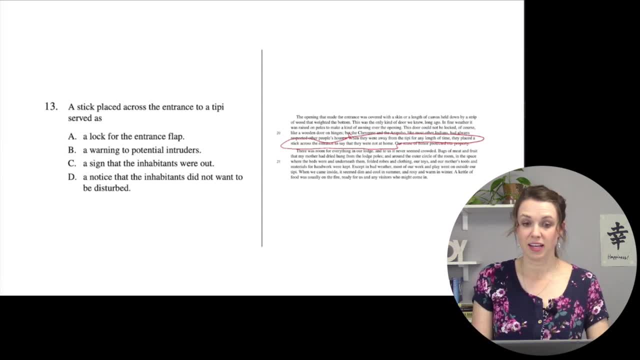 they placed a stick across the entrance to say they were not at home. So there's our answer. right, It was a sign that the inhabitants were out. So a lot of times you can if you have an idea of what the questions are. 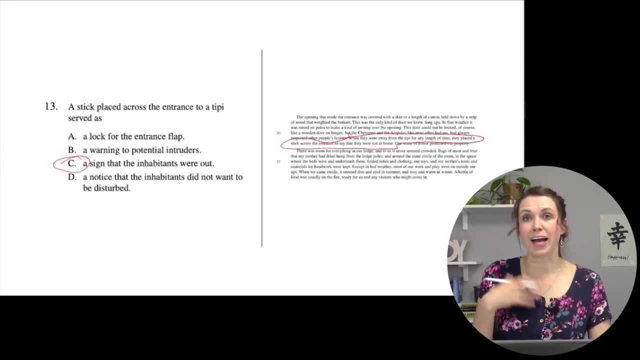 like in this case, if we would have read the question before we actually read the article, we would have known, oh, that's one of the questions, right, And we would have been able to answer it very easily. but luckily we were able to find it fairly quickly. 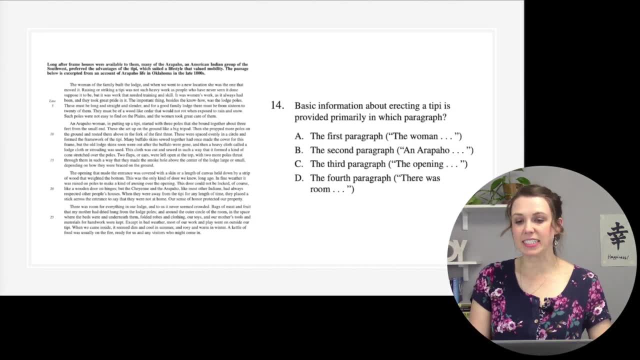 14, basic information about erecting a teepee is provided primarily in which paragraph? Okay, so you gotta know what this word here means: right Erecting. so that means putting up right. So which paragraph talks about how to put up a teepee? 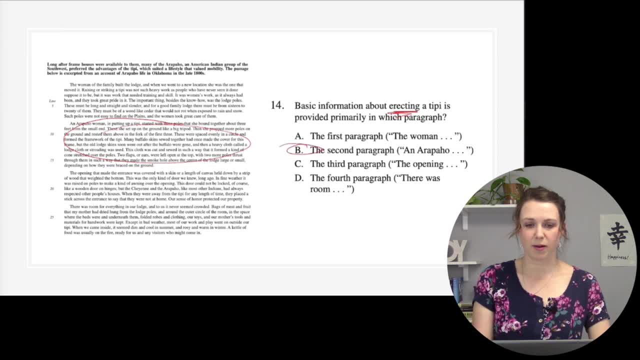 Definitely this second paragraph here, right. It talks about the poles, or I guess the poles are a little bit in the first one. It tells you how to put the poles together, what to do, that sort of thing. That one teaches us how to put up the teepee. 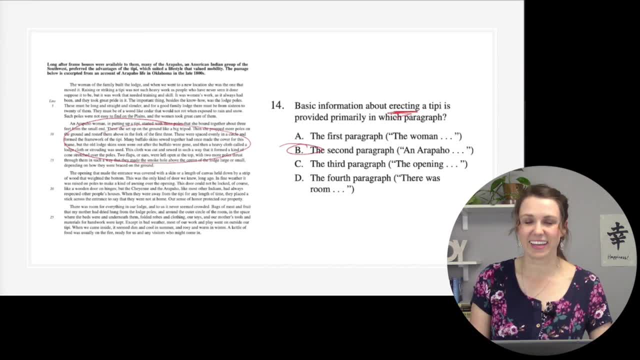 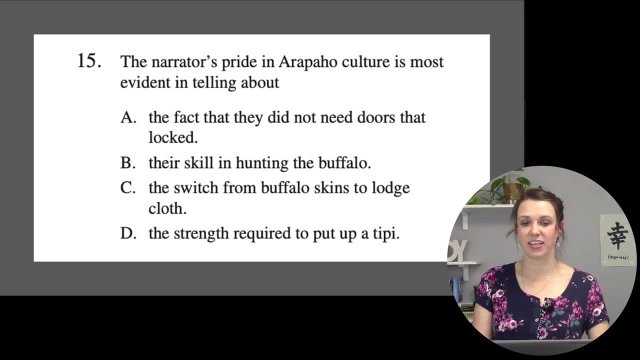 Are you ready to do this? Ready to put up a teepee? I think I might need a little more practice. The narrator's pride in Arapaho culture is most evident in telling about the fact that they did not need doors locked. It did talk about that, right. 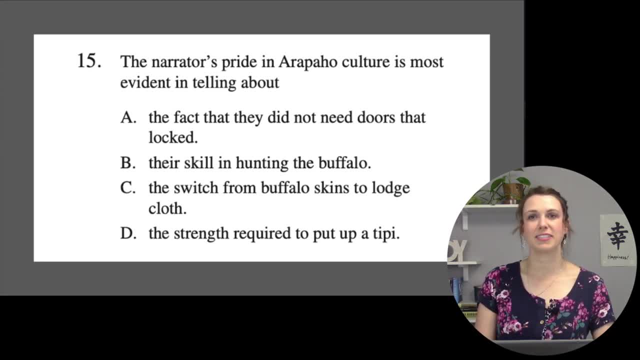 It talked about how there was a sense of pride. They just put the stick in front and that means that they're home and people respected that right. It sounds like he's really proud of that- Their skill in hunting the buffalo. 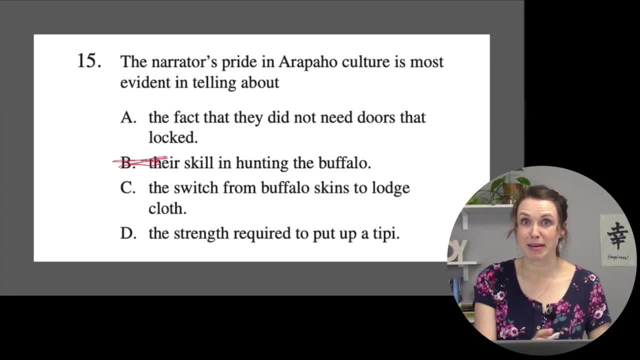 Did it talk about that at all? No, it talked about how the buffalo were becoming more scarce. right The switch from buffalo skins to lodge cloth. Do you think he takes a lot of pride in that? Not so much The strength required to put up a teepee. 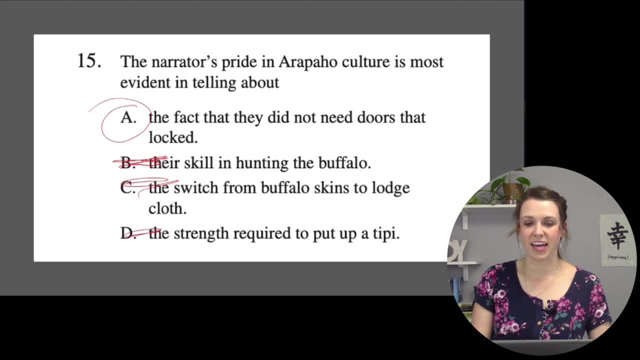 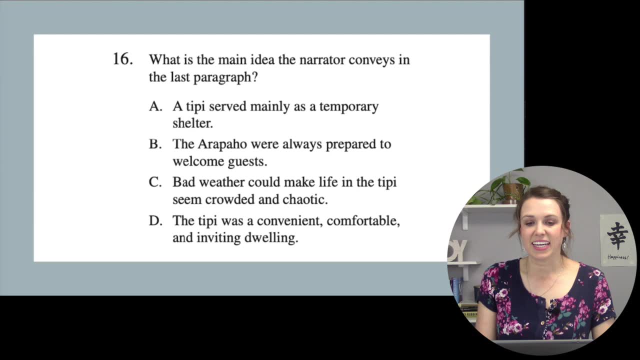 He's not really showing that either, right? So the answer here is definitely A. We don't have to lock our doors, We just put a stick across our door. What is the main idea the narrator conveys in the last paragraph? I don't have this paragraph showing. 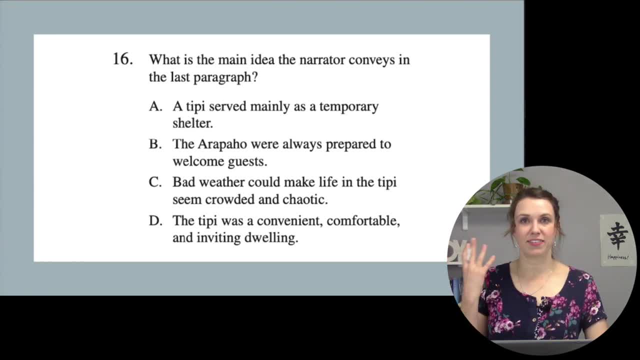 but in this paragraph it really talks about what the inside of the teepee is like. right, It talks about how dried fruit and meats are being hung, how there are the beds with the robes and the clothes, and also how people don't really you know. 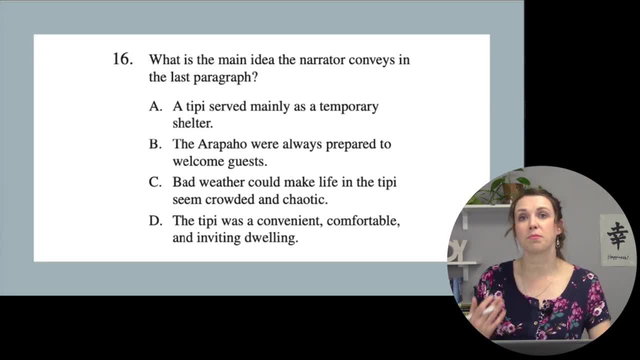 spend much time in the teepee. Most of their work and their play is done outside, and then the teepee is nice and cool in the summer and warm and toasty in the winter. right, So that's really what it is talking about. 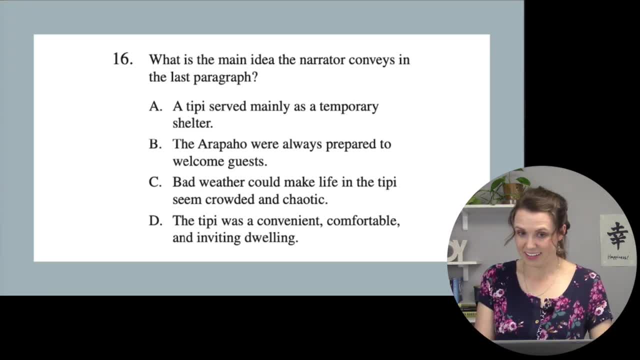 So, that being said, A the teepee served mainly as a temporary shelter. Doesn't really talk about how it's like a temporary right. It talks about the purpose of it. The Arapaho were always prepared for the winter right. 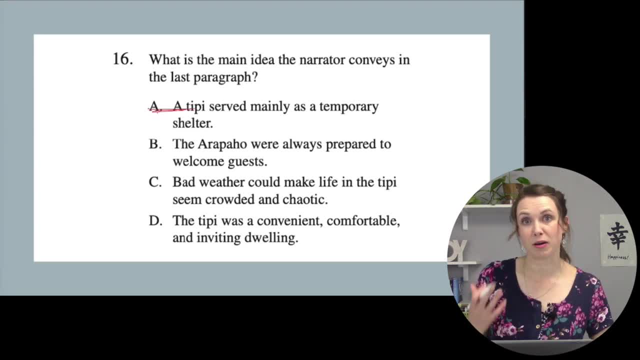 The Arapaho were always prepared for the winter right. The Arapaho were always prepared to welcome guests. It did mention welcoming guests, but that was just a supporting detail of the paragraph. that wasn't the main idea. Bad weather could make life in a teepee. 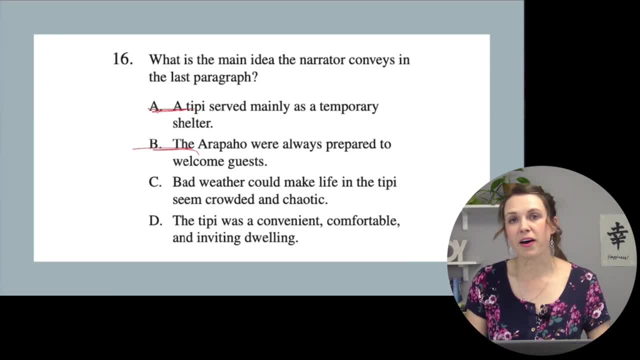 seem crowded and chaotic. It talks about how they always felt like there was room right, not that it was crowded and chaotic. So the teepee was a convenient, comfortable and inviting dwelling. Yeah right, They're comfortable in that teepee. 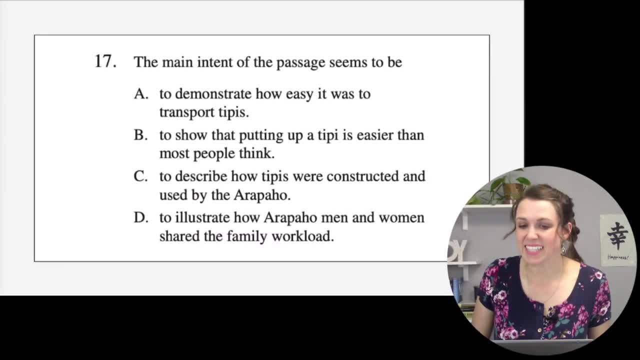 They're comfortable in that teepee. They're comfortable in that teepee Right. The main intent of the passage seems to be so. why did they write this right? So to demonstrate how easy it was to transport teepees. Didn't really talk a whole lot. 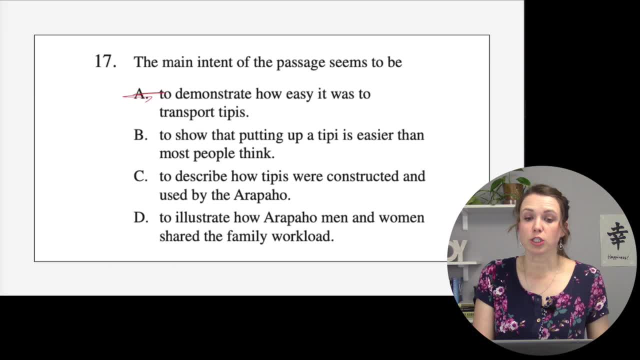 about the transportation right. B, to show that putting up a teepee is easier than most people think. Well, I have the one paragraph about putting up a teepee, but the whole passage wasn't really about that, right? But the whole passage wasn't really about that, right. 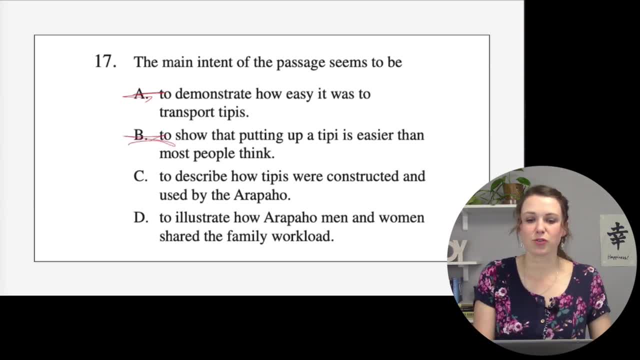 But the whole passage wasn't really about that. right to describe how teepees were constructed and used. There we go: How they were built and how they were used. That was really what it focused on. right Or D to illustrate how Arapaho men and women shared the family workload. 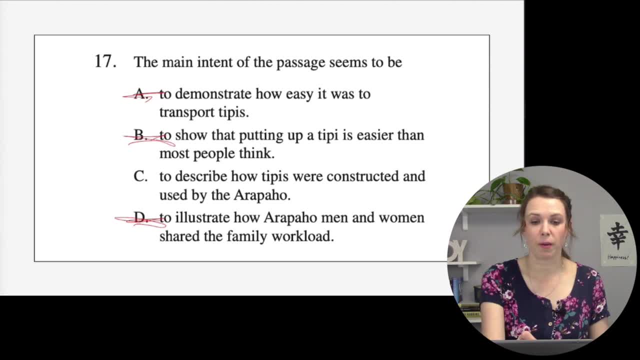 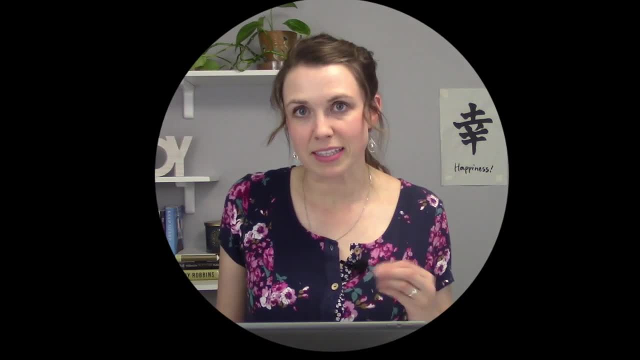 It didn't really talk about the workload of men, right? It really focused on women. So the answer is D. So now we're moving on to our poetry section, And poetry can be a little bit tricky And I just want you to do your best. 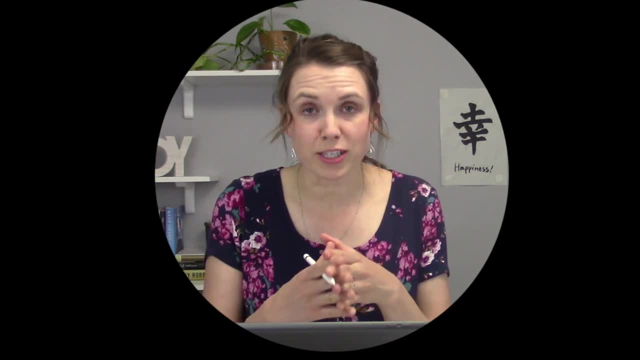 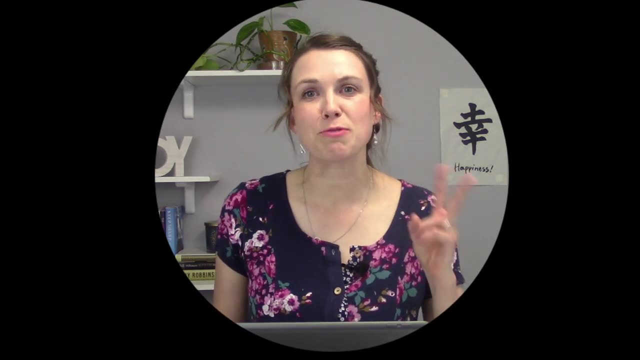 I actually have a couple poetry videos that you might consider watching so that you really have a thorough understanding of poetry. But just do your best, okay. So we've got two poems here that we're going to be going over. So for this first poem, I'm going to start off by doing a little surveying. so I know what's going on. So it says: For the chicken eggs to hatch, whether they are brown or white, two cats Conditions are necessary. They must be fertile and they must be kept at a constant temperature of 99.5 degrees Fahrenheit. 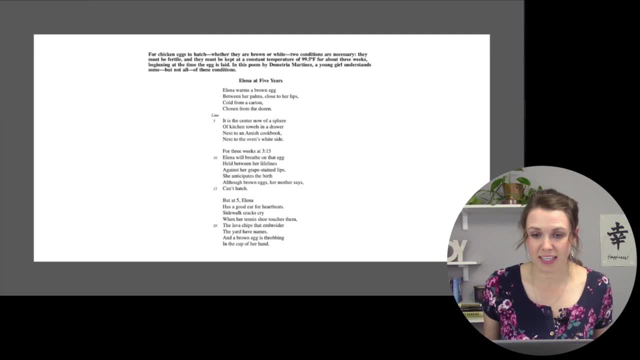 for about three weeks, beginning at the time the egg is laid. In this poem by Demetria Martinez, a young girl understands some, but not all of these conditions. So we have Elena at five years old. So with poetry, I like to just read, maybe like the first line of: 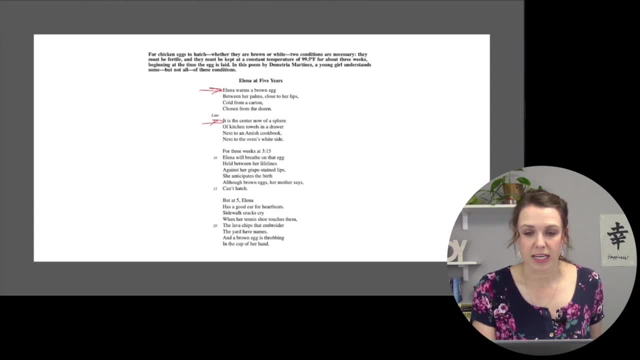 each little stanza. when I'm just surveying, Elena worms a brown egg. It is at the center of center now of a sphere, for three weeks at 315.. But at five, Elena. Okay, so I have a general idea of what's going on. 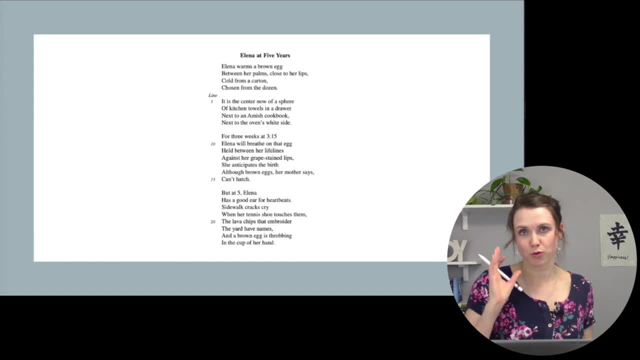 And I'm going to. normally I would read the questions, but I'm just going to go straight to the poem. So now I normally just take a quick look at the questions, but in this case we're just going to go right to our poem. 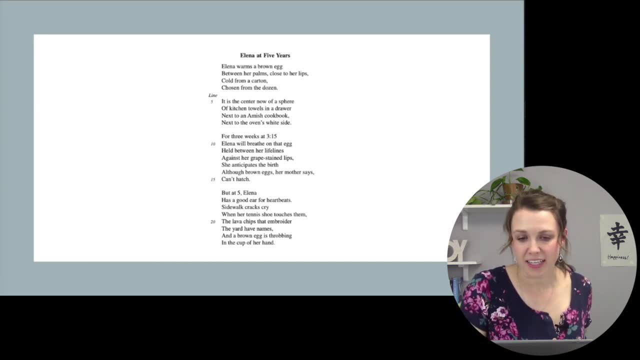 Elena at five years. Elena warms a brown egg Between her palms, close to her lips, cold from a carton chosen from the dozen. It is now. it is the center now of a sphere: A kitchen towel in a drawer, next to an Amish cookbook, next to an oven's white side. 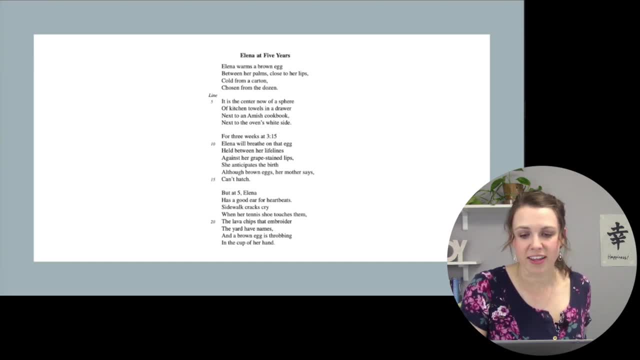 For three weeks, at 315,, Elena will breathe on that egg held between her lifelines, Against her great interfere, her grape-stained lips, She anticipates the birth, although brown eggs, her mother says, can't hatch. But at five, Elena has a good ear for heartbeats. Sidewalk cracks cry. Winter tennis shoes touch. 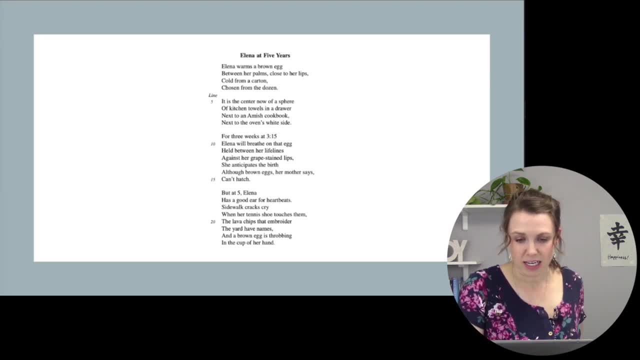 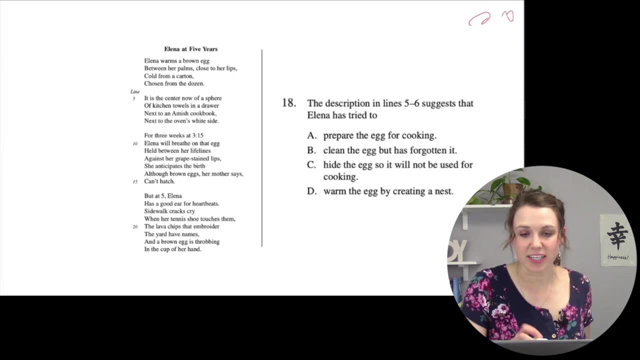 them: Lava chips that embroider the yard, have names and a brown egg is throbbing in the cup of her hands. The description, lines five and six, suggest that Elena- so five and six- has tried to prepare the egg for cooking. Oh heavens, no, She's trying to hatch the egg right. Clean the egg, but 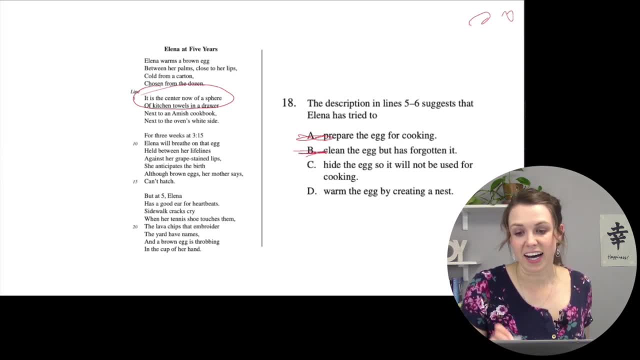 has forgotten it. Oh, she hasn't forgotten it. Hide the egg so it will not be used for cooking. No, she's not trying to hide it, right? She's trying to warm the egg by creating a nest, Isn't she? 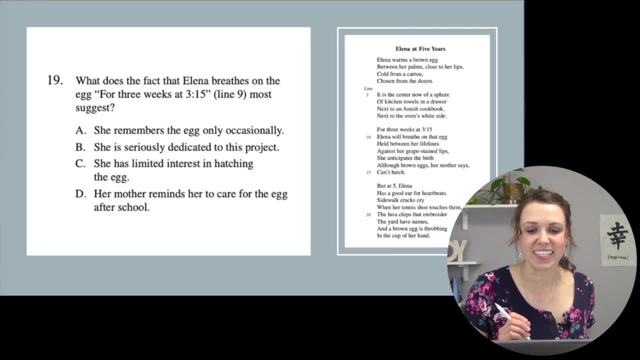 sweet. Okay. what does the fact that Elena breathes on the egg for three weeks mean? She's trying to warm the egg by creating a nest, Isn't she sweet. She speaks at 315 in line, nine most suggest. So she remembers the egg only occasionally. No, 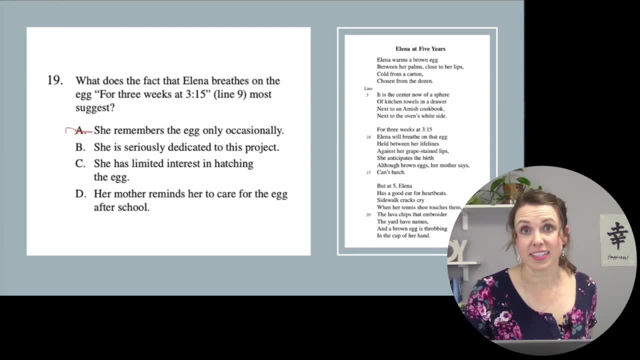 she remembers it every day. 315, right, She is seriously dedicated to this project. Yes, she is. She has limited interest in hatching the egg and she's not. it's not limited, right? Her mother reminds her to care for the egg after school. Is her mother reminding her? 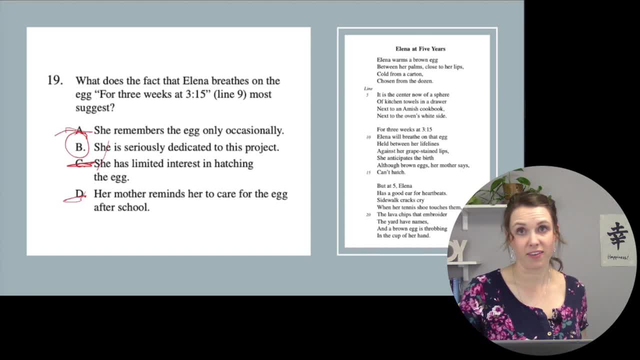 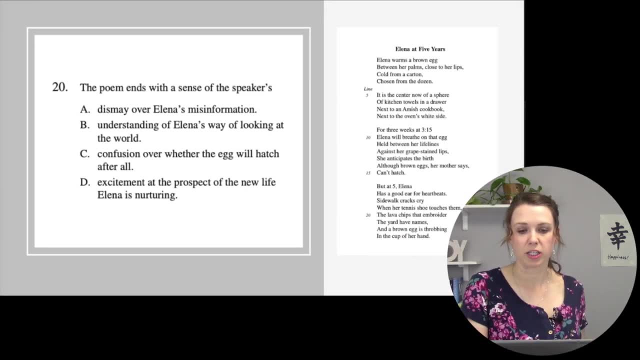 No right, She is so dedicated. She's like I've got this 315, three weeks, I can do this, Okay. the poem ends with the sense of the speaker's dismay over Elena's misinformation. No, it's like describing this little five-year-old in her. 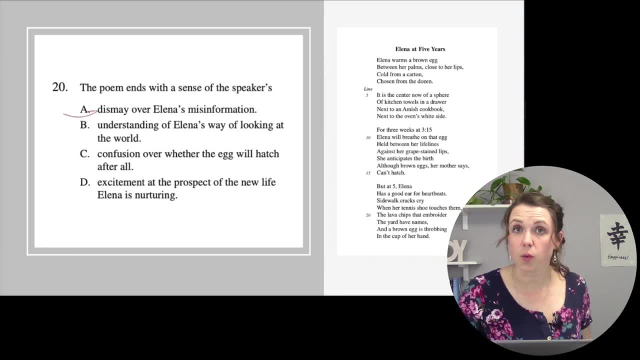 imagination, right, Understanding Elena's way of looking at the world. Yes, right, She can hear the sidewalks crack. She can name the lava chips. right, Five-year-olds have such vivid imaginations. So that's our answer here. but let's look at the other ones. 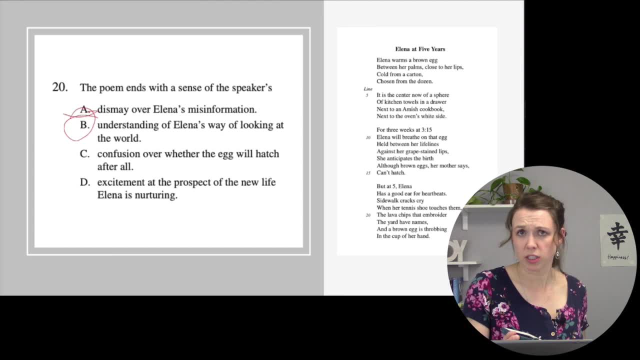 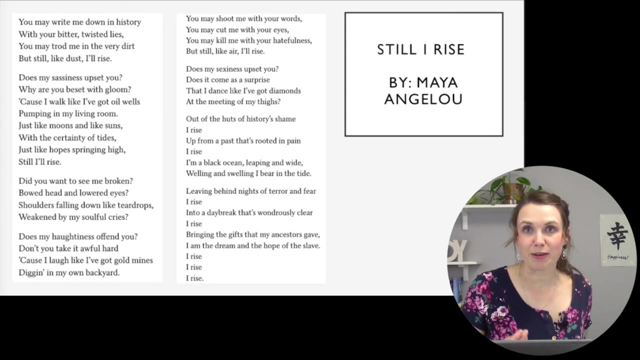 Confused over whether the egg will hatch. No, she's convinced this egg is going to hatch, right Excitement at the prospect of new life that she is nurturing. Yes, she's excited, but it's definitely her way of understanding things. So we're going to read a different. 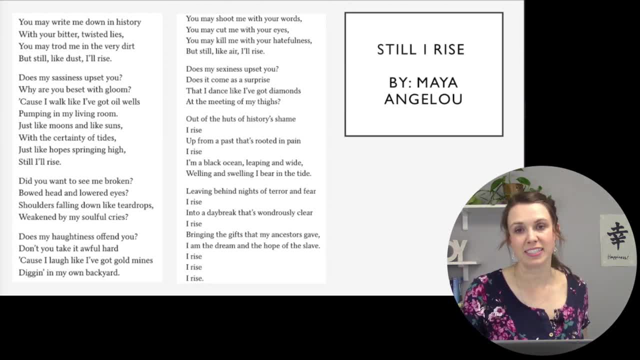 poem now, and this one actually does not go with the high set practice test. This is a poem that is a pretty powerful poem, written by- I don't even know how to say her name- Maya Angelou, And she was an African-American woman- and it's definitely a powerful poem. 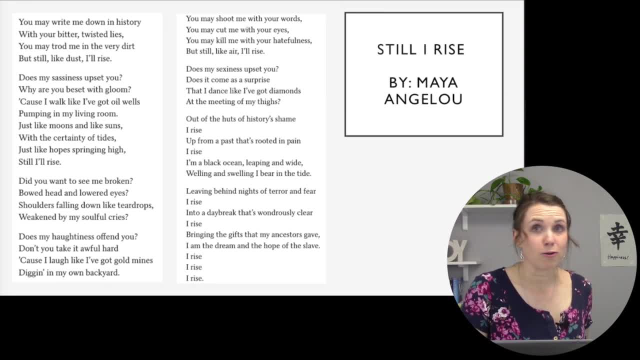 just sort of illustrating how she can be powerful, and despite the world of racism. So we're going to take a quick read of the poem and then answer a few questions. You may write me down in history with your bitter, twisted lies. You may trod me in the very dirt, but still, like dust, I'll rise. 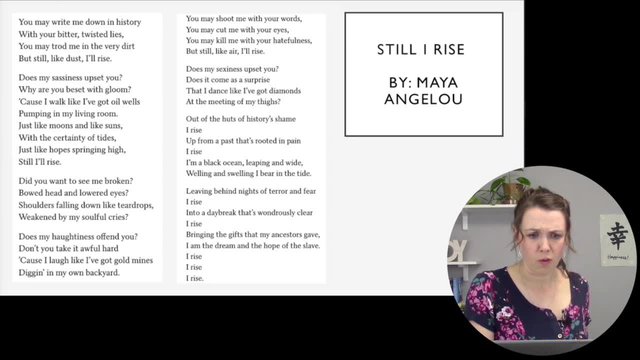 Does my sassiness upset you? Why are you besieged with gloom? Because I walk like I've got oil wells pumping in my living room, just like moons and like suns, with certainty of tides, just like hopes springing high still. 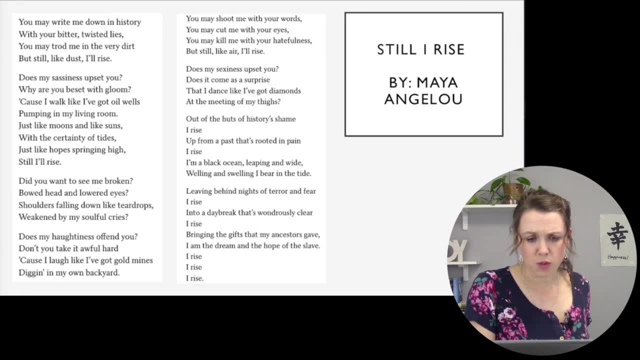 I'll rise. Did you want to see me broken, bow-headed and lowered eyes, shoulders falling down like teardrops, weakened with my sorrowful cries? Does my haughtiness offend you? Don't you take it awful hard, Because I laugh like I've got gold mines digging in my own backyard. 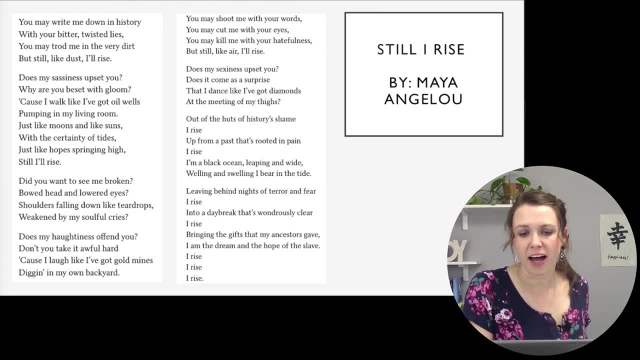 You may shoot me with your words, You may cut me with your words, me with your eyes. you may kill me with your hatefulness, but still, like air, I'll rise. does my sexiness upset you? does it come as a surprise that I dance like I've got diamonds at the meeting? 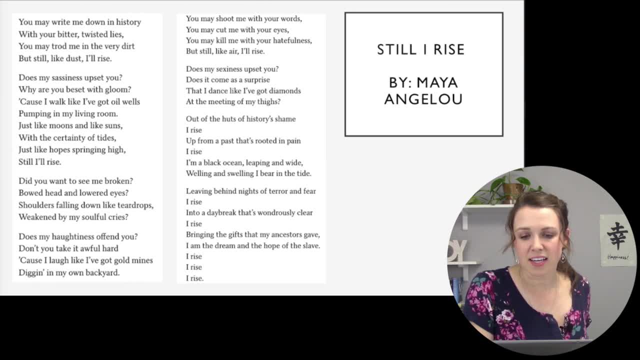 of my thighs, out of the huts of history's shame, I rise up from the past that's rooted in pain. I rise. I'm a black ocean, leaping and wide, welling and swelling. I bear in the tide, leaving behind nights of terror and fear. I rise into a daybreak that's wondrously clear. 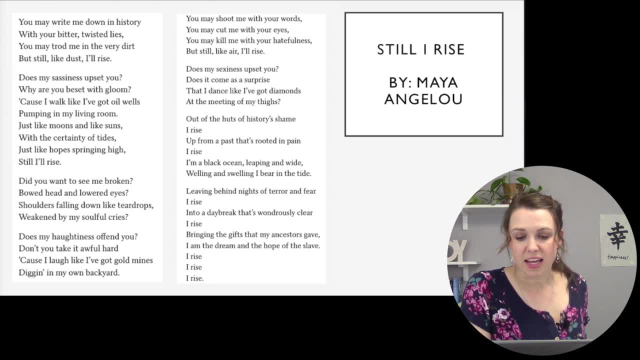 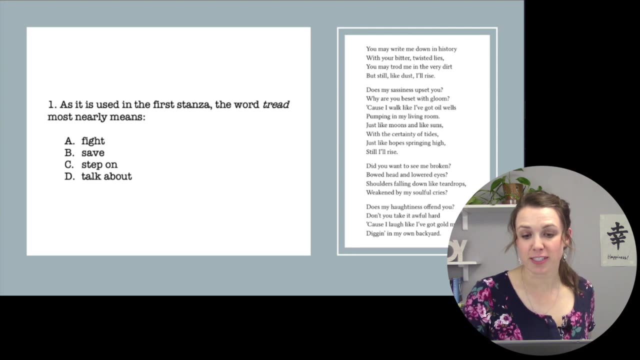 I rise, bringing the gifts that my ancestors gave. I am the dream of hope and the hope of the slave. I rise, I rise, I rise. as it is used in the first stanza, the word tread most nearly means it's actually not tread, it's actually trod. you can see in the first, the third line there, but uh, my pen is not working. 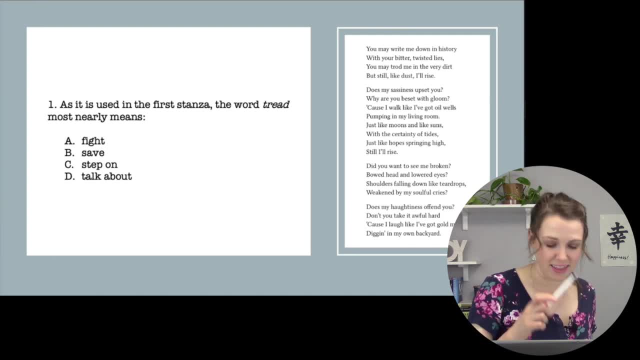 anymore. so I can't really cross off our mark answers, but that's uh, that's okay, we're just gonna go with it. so, trod, does it mean to fight? so let's look at it. you may trod me in the very dirt, right. so, trod, do you fight on dirt? 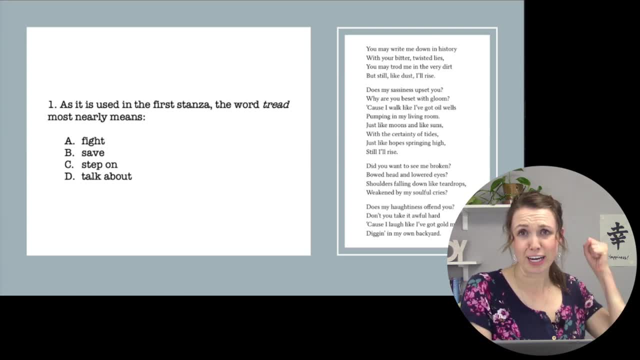 do you save dirt? save the dirt. do you step on right? you may step on me in the very dirt right. I mean here it's kind of talking about how this person is being belittled, right still like dust, right. so you may step on me in the very dirt right. so you may step on me in the very dirt right. 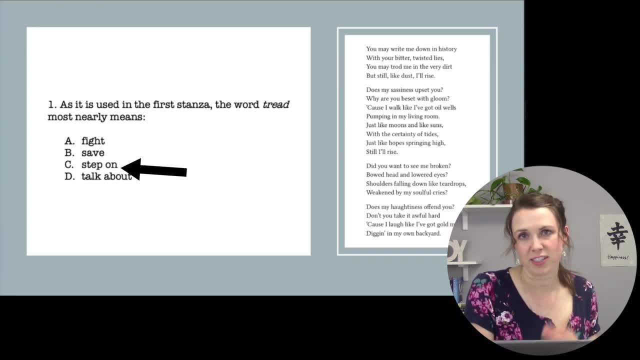 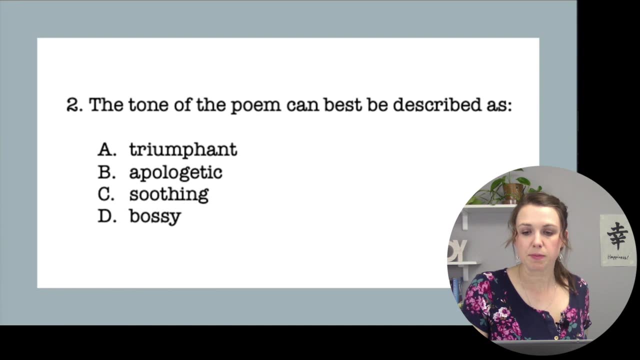 so it's like: you know, step on me, but I'm gonna rise, you're not gonna stop me, right? and so the answer here is C. the tone of the poem can best be described as triumphant. yeah, right, she's like: yes, there, you know, I don't care what happens, I will rise, I'm gonna do great things, right? we as 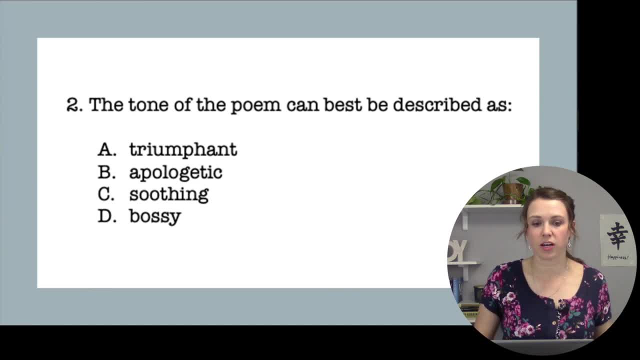 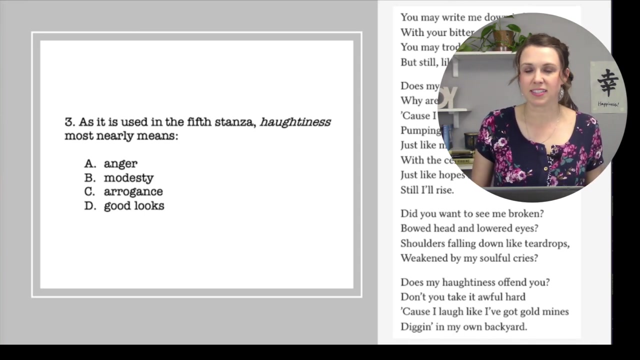 a society are gonna do great things right. that's what she's talking about. is she apologetic? oh I'm sorry, right? no, she's unapologetic like. this is who we are. we're gonna do great things right. soothing bossy, no, so definitely a. as used in the fifth stanza, haughtiness most nearly means so again. 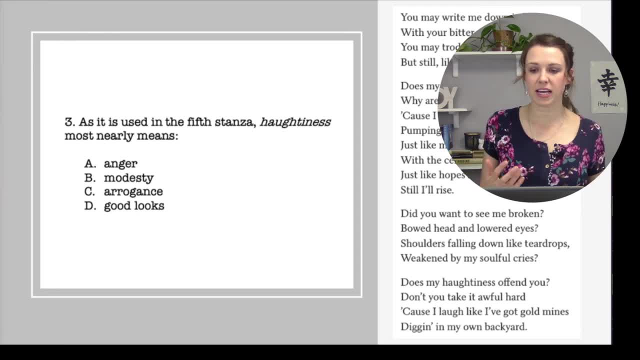 normally the stanzas will be labeled, but in this case it's not. but you can see haughtiness is right down there at the bottom. so it says here: does my haughtiness offend you? don't? you don't take it awful hard, right? so, haughtiness, is it anger? is she angry? it's not really showing a lot of anger, right, is she being? is she trying to be modest? no, arrogant, yeah, she's like, does my arrogance offend you? like I'm like I don't really care, right, that's kind of what she's going on. oh, good looks, do her good looks offend you? no, so, 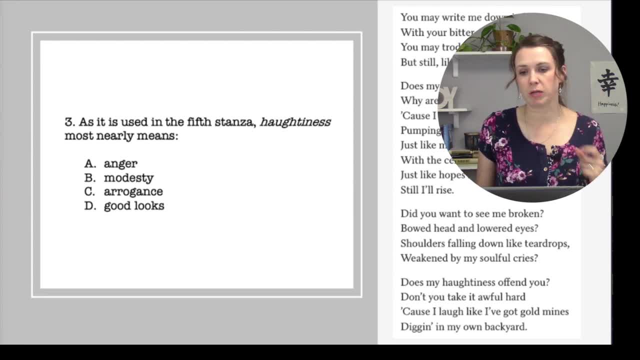 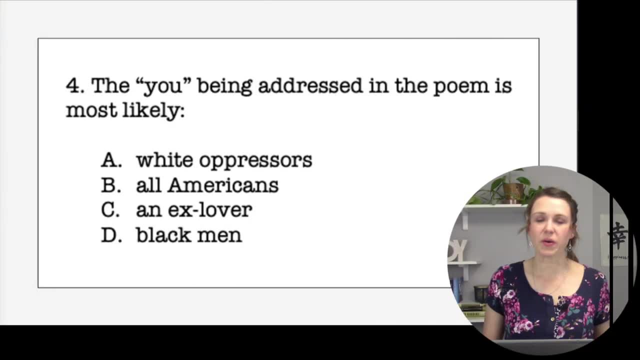 it's definitely arrogant, right she's? she definitely is being arrogant within this, within this poem, but does it offend you, okay? so she's talking about you? who is you? now, keep in mind this is a black woman who is writing this about racism, right? so the you is most likely white oppressors. so, yeah, right, she's talking about white people that are. 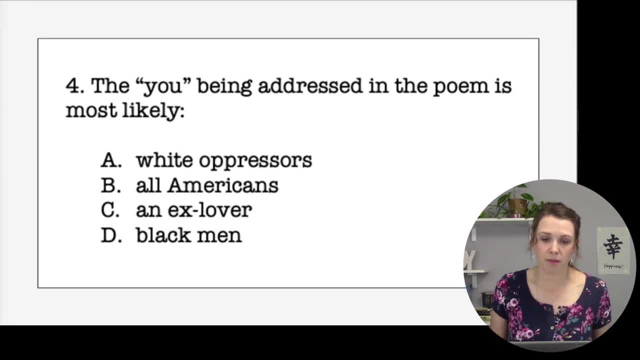 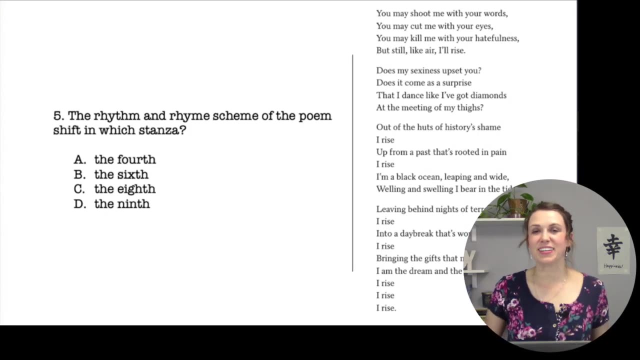 right, ok, I, this stanza is just like a paragraph. usually it's separated it within lines, And so I don't have the entire poem here, but I just wanted to show you this part right here. So it says: if you look at the very end of the first stanza, we have eyes and then 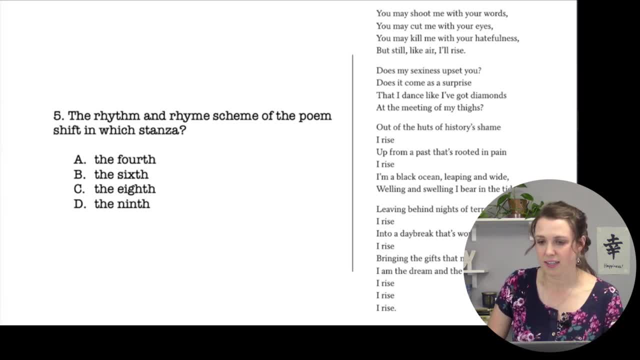 the last line says: rise, eyes rise, And then we have surprise. and then thighs right. But then it starts to change it up a bit. right Out of the huts of history's shame, I rise Up from the past that's rooted in pain. I rise So that right there it really doesn't have the same rhythm. 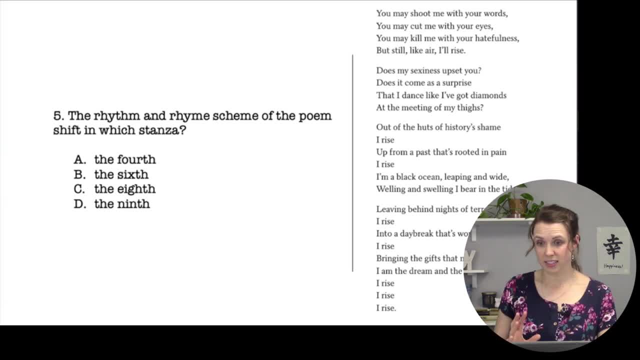 that the rest of the poem has, And also it doesn't have that same rhyme scheme. And so, even though you can't tell this, because the whole poem isn't included, it would be C, which is the eighth stanza. This here's the eighth stanza, even though it looks like it's. 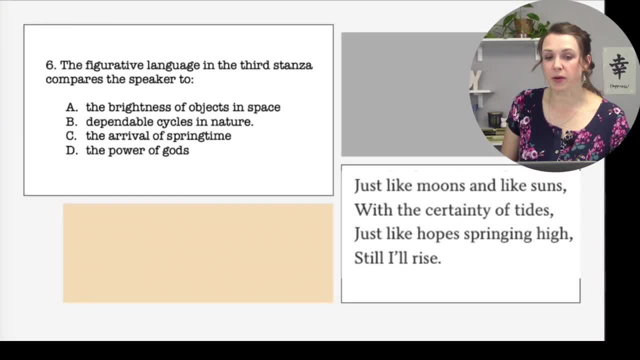 the third stanza. it's actually the eighth. The figurative language in the third stanza compares the speaker to. so here I've got the third stanza. just like moons and like suns with the certainty of tides, just like hopes springing high, still I'll rise. 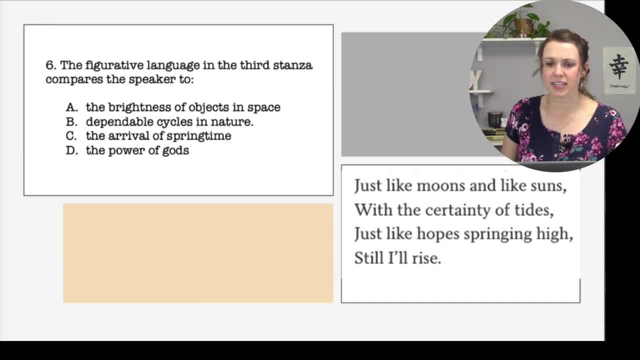 Right. So what is this kind of referring to, right? Is it brightness of objects in space? Is that what it's talking about, right? Notice how it says the certainty of tides. It's not really talking about the brightness, right, Dependability. 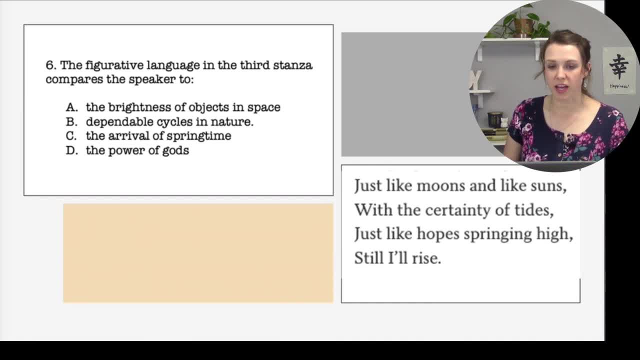 Certainty is like dependable right, Dependable cycles in nature, The moon, the sun, the tides. very certain, very predictable right. So that's the answer there. B. But let's look at C and D: The arrival of springtime. 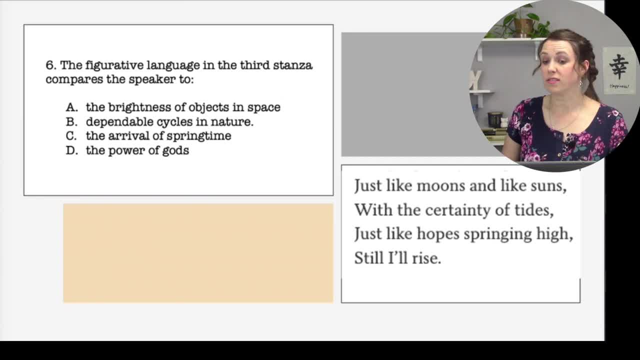 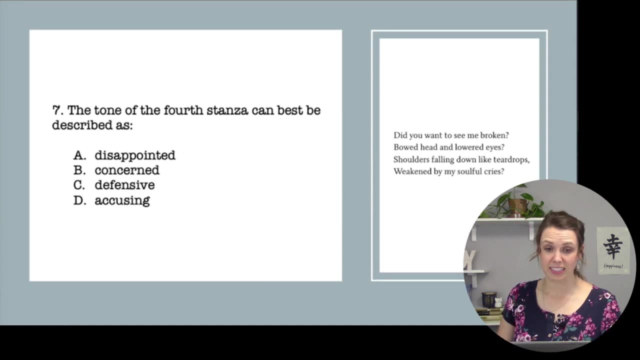 So it says springing high, but it's not really talking about see the power of gods. No, it's not talking about the power of gods, right? It's talking about that dependability. Okay, So the tone in the fourth stanza can be described as: so let's take a look at it. 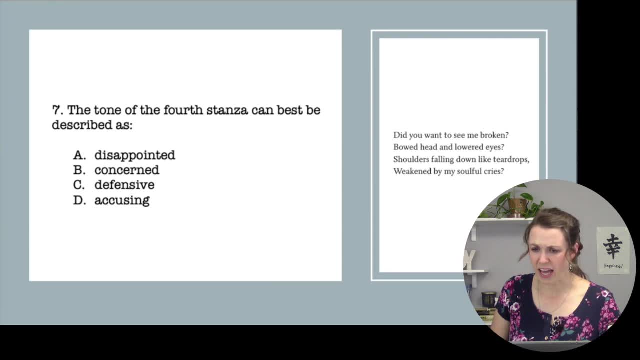 Did you want to see me broken, bowed head and lowered eyes, shoulders falling Down like teardrops, weakened by my sorrowful cries? So is it disappointed? Not so much because it's saying: did you want me to feel like this? 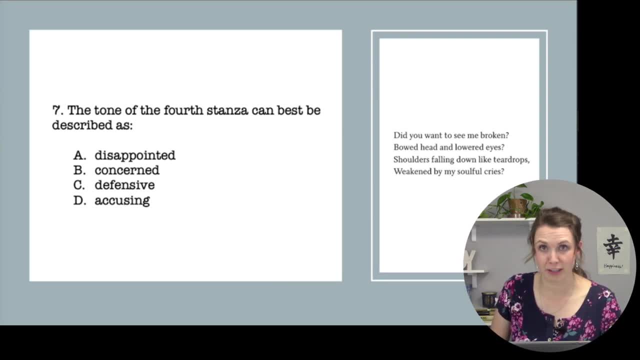 Right, Remember, she's arrogant, right. This poem has arrogance in it, Concerned, not really defensive. There's a little bit of defensiveness going on, but accusing. look at that. She's like: did you want me to be like this? Right, She's very. 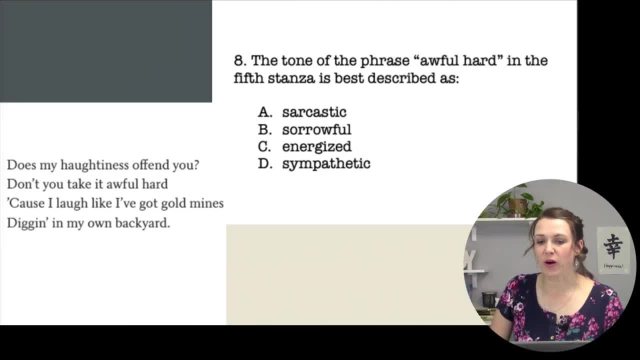 very accusing right. So D is our answer. The tone of the phrase awful hard in the fifth stanza is best described as: so does my haughtiness offend you, Don't you take it awful hard? So is she being sarcastic? Absolutely Right. 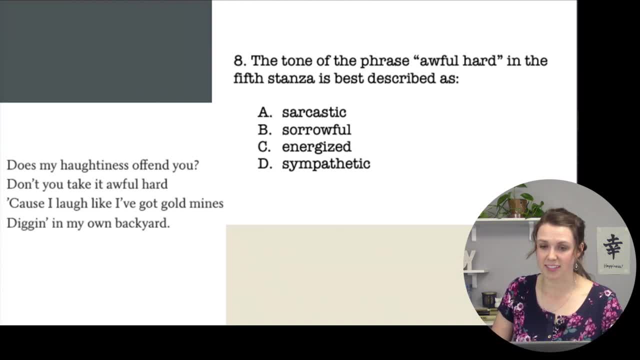 We've got that arrogance again, definitely showing sarcastic tone right. Sorrowful, Not really. Energize, Is she energizing? Does my haughtiness offend you? No, Sympathetic, Not really. So the answer is A. I know this is a reading test, but let me throw in some grammar. 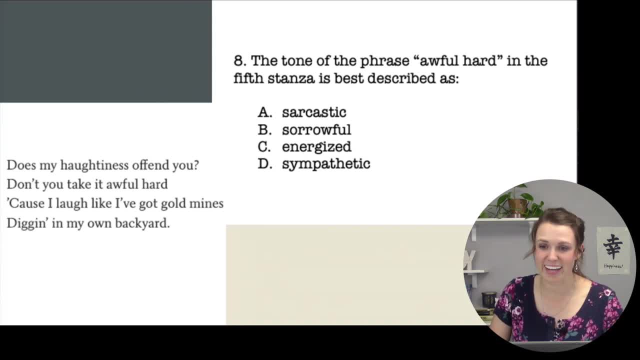 Awful hard is actually grammatically incorrect. It should be awfully hard. So awful is described, is an adverb in this case, And so it has to end in L-Y: awfully hard. So you know. reading in, reading in grammar: 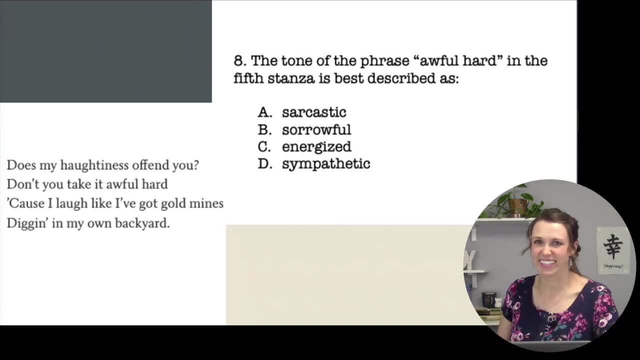 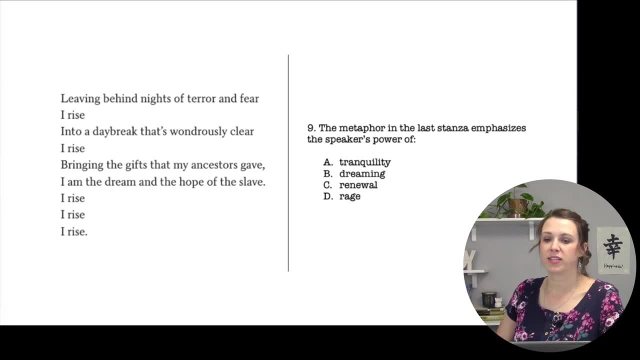 hand in hand reading and writing, So I had to chime that in. Okay, The metaphor. So a metaphor is a comparison, right? The metaphor in the last stanza emphasizes the speaker's power of. so let's see here It says: leaving behind nights of terror and fear. 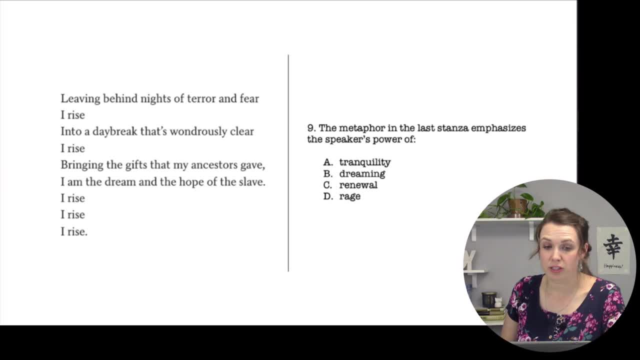 I rise Into a daybreak. That's wondrously clear. I rise Bringing in the gifts that my ancestors gave. I am the dream and the hope of the slave. I rise, I rise, I rise Right. Tranquility. Is it peace, Tranquility? 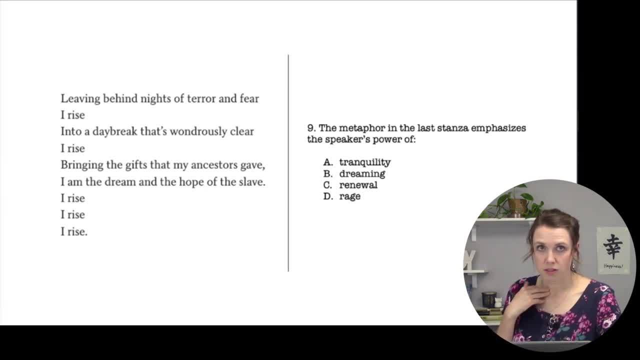 and peace. Not so much Dreaming- She seems like she's a little more powerful than it just being a dream right. Renewal, Yes, I rise, I rise. right That's. that's a sense of renewal right. 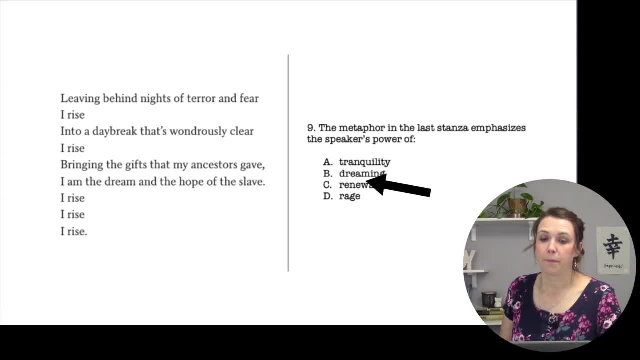 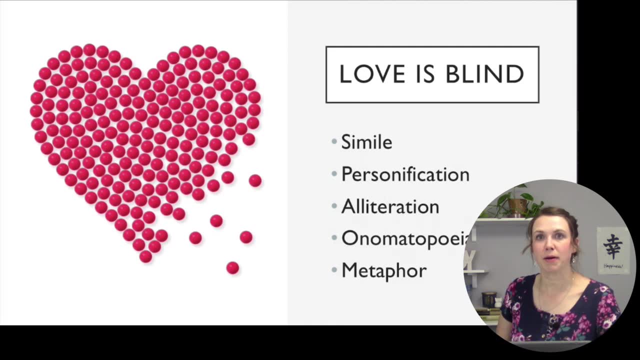 Rage. I mean there's rage within it, but it definitely is more of that renewal. Okay, I needed one more question because I promised 30 questions. So love is blind. Is that a simile, Personification, alliteration, onomatopoeia or metaphor? Let me do a quick. 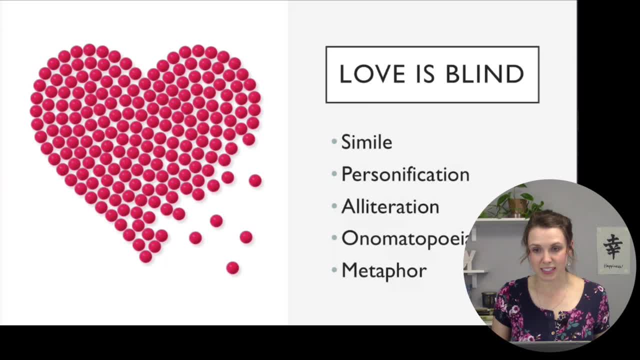 review of these terms. Simile is a comparison using like or as or as if. Notice how it says is Not like as or as if, So it's not a simile Personification. That is when you're comparing maybe an object or an animal or something to human-like characteristics or characteristics. 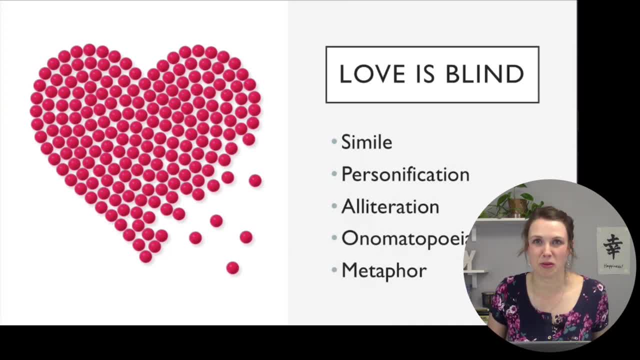 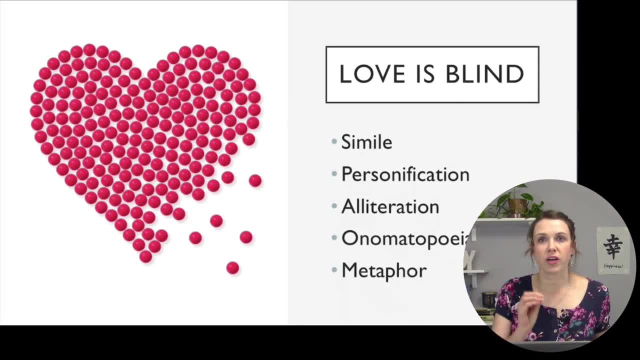 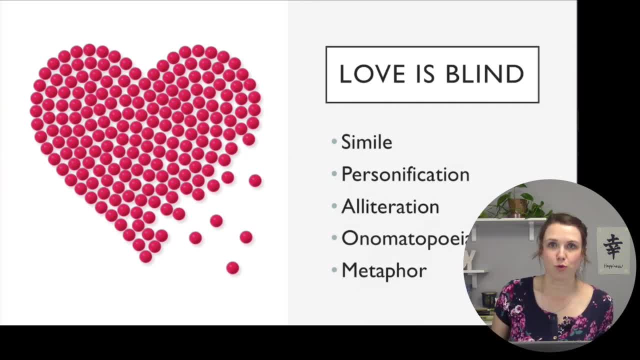 Onomatopoeia would be words like roar, click, hiccup right, Words that actually sound like they are. So the the name of the word is how it sounds And metaphor is a comparison. just like simile, except it does not use like as or as if. 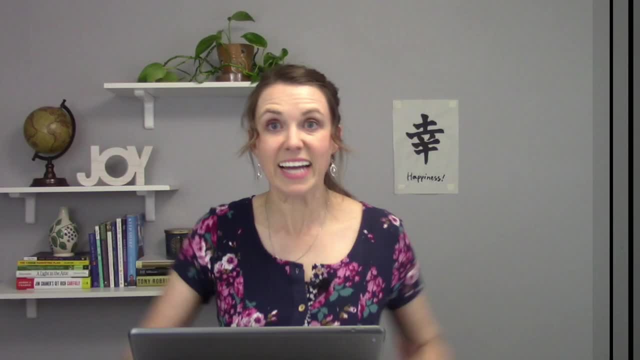 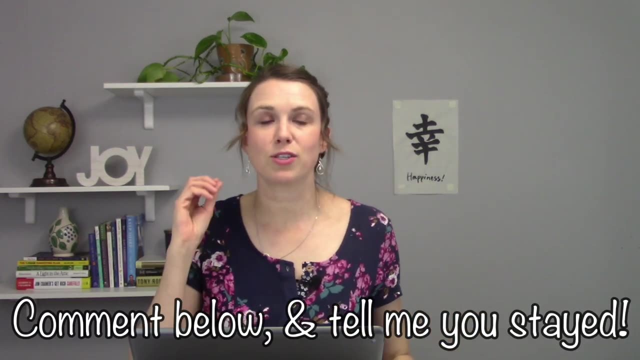 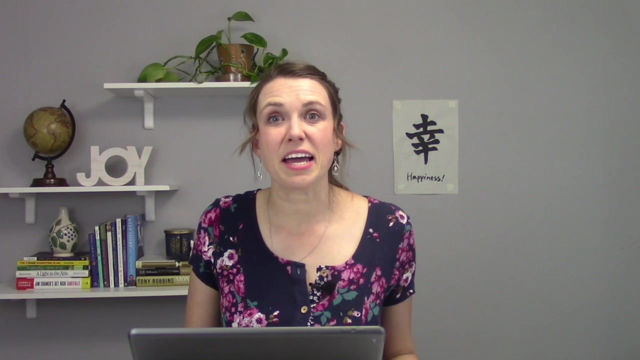 So love is blind is a metaphor. Guys, we're done another long video And if you stuck around, comment below and tell me because you're so committed- I mean, these videos that I've got here are long, but being a practice test, it really, really helps you. 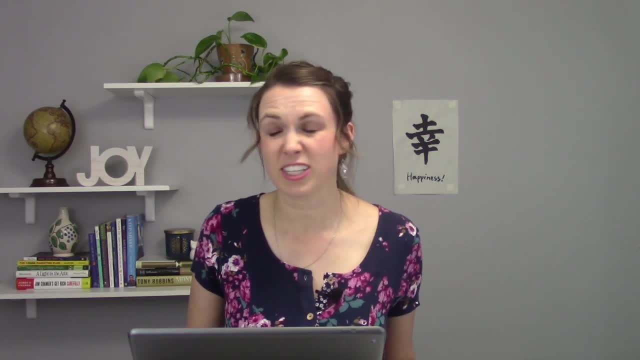 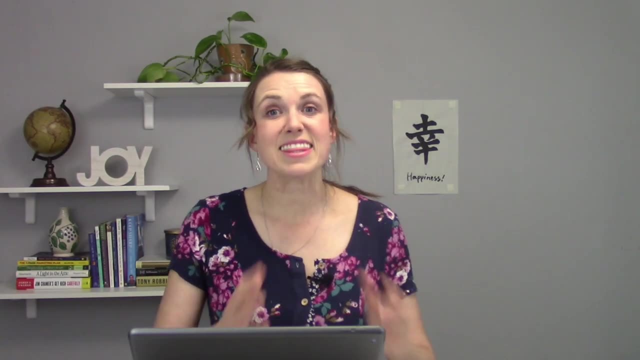 to stick with the whole thing and I know you're gonna do it. You're gonna get your high set, you're gonna get your GED because you're working so hard. So, like I said, comment below And, guys, thank you so much for this difference.